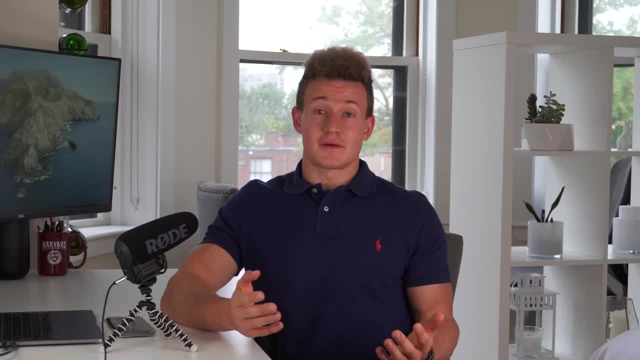 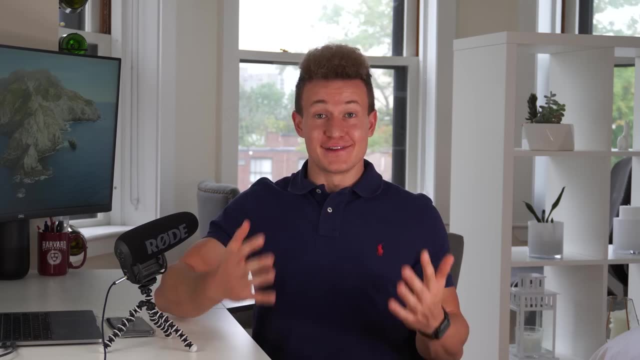 Sometimes it's because your teacher is doing a very bad job at explaining a concept, but often the concepts are just so complicated that it's nearly impossible to immediately understand them after hearing them for the first time. In this video, I'm going to show you a 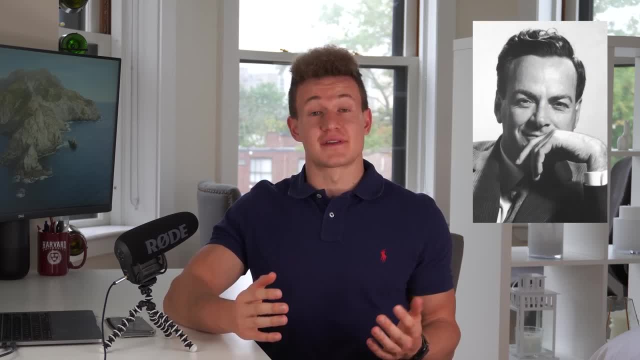 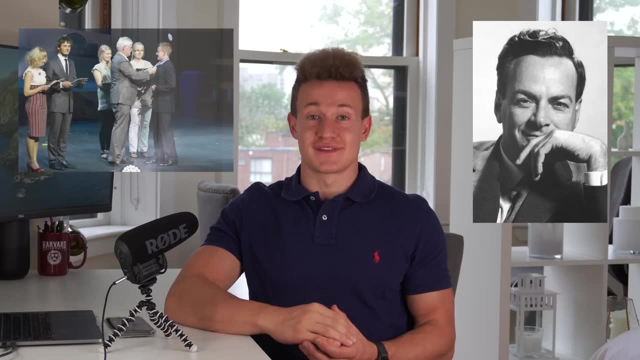 strategy used by Richard Feynman, one of the greatest physicists of all times, for solving very complex problems. I'm also going to show you how I use this strategy for winning a medal at the International Physics Olympiad. Before we get started, make sure to subscribe to my channel. 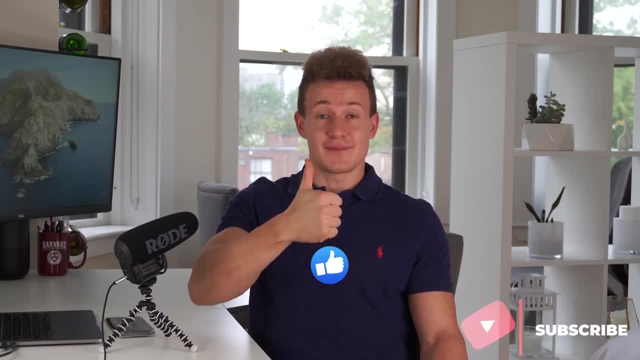 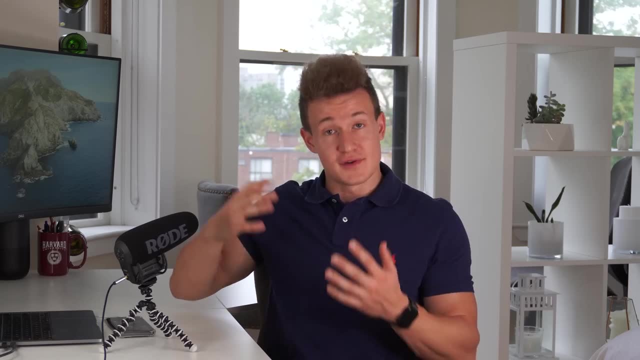 down here for some more tips and tricks, And while you're there, you can also hit the like button to push the YouTube algorithm. Feynman's strategy can be applied to almost any kind of problems, from simple mathematics all the way up to differential geometry and even some business. 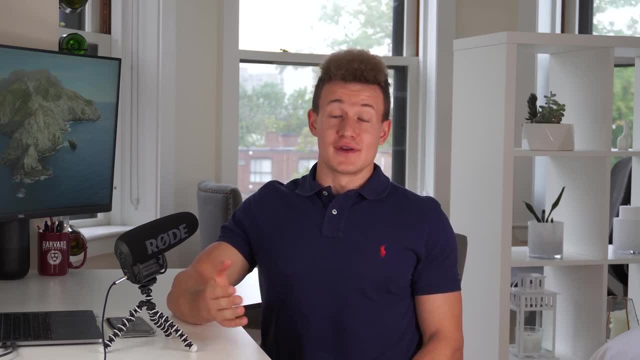 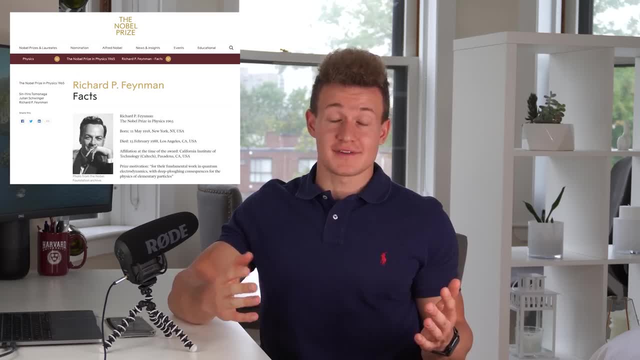 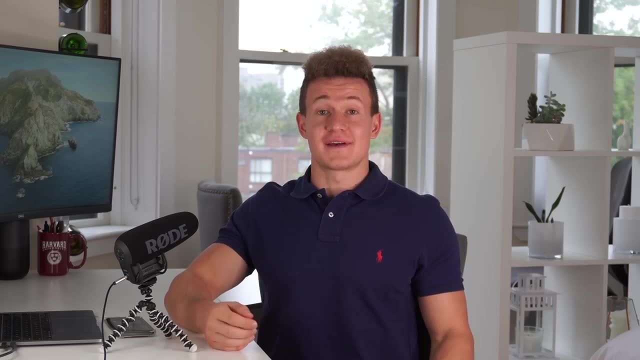 and he won the Nobel Prize in Physics. and he won the Nobel Prize in Physics in 1965 for his work in quantum electrodynamics. and, little fun fact, he walked these very corridors as a student at MIT. But what made him so special, compared to all the other great scientists, was his unique. 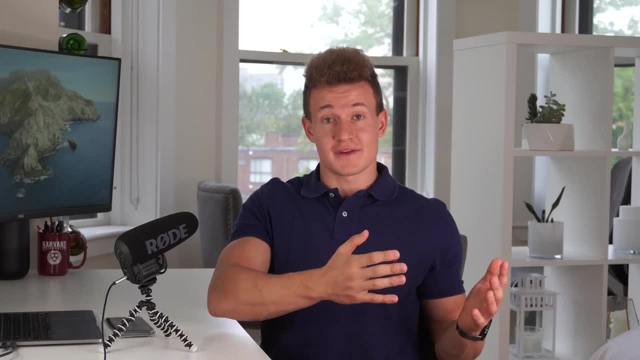 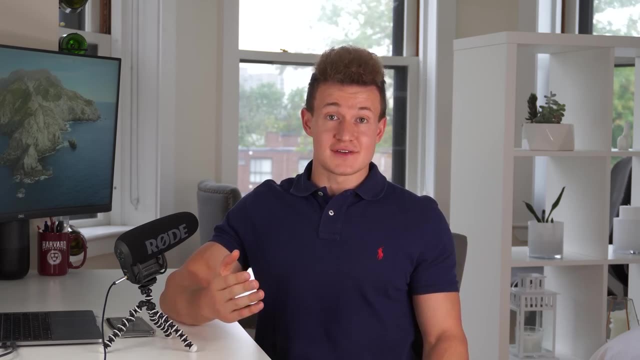 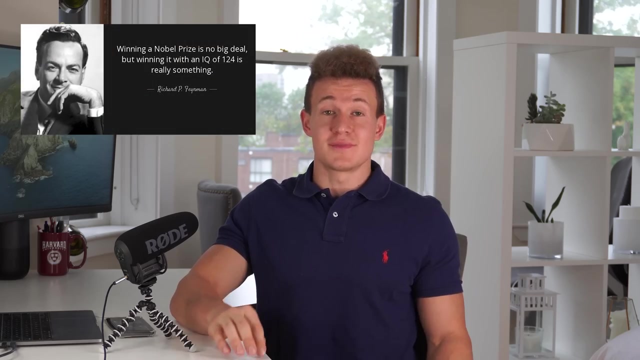 personality and incredible ability to understand complex concepts and solve difficult problems. Surely Feynman was a very smart guy, but I'm very convinced that his intelligence alone played only a minor role in his success. According to himself, he only had an IQ of 124, which means that roughly 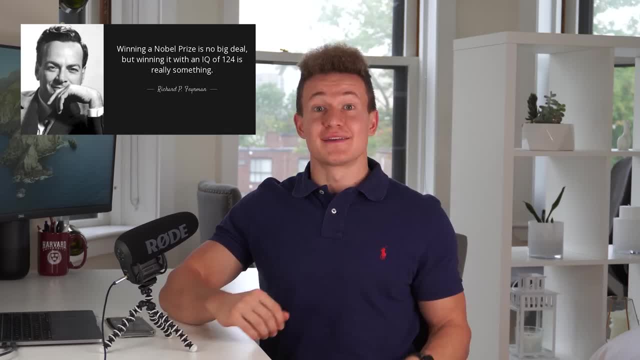 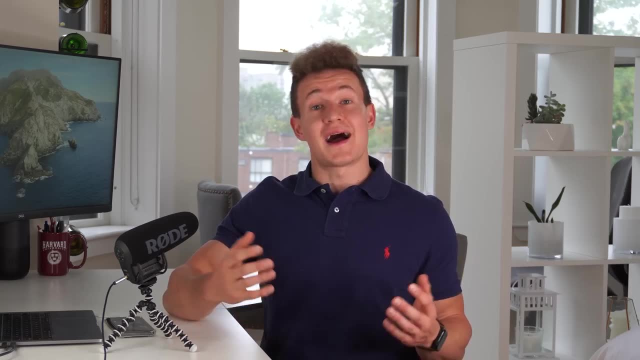 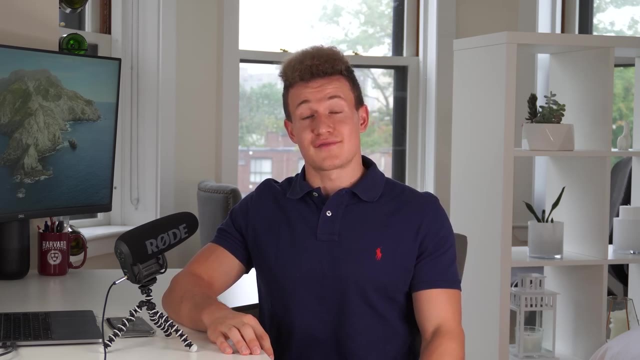 5% of the world population is actually more intelligent than him. So if Feynman could revolutionize physics with an IQ of 124 just by using clever problem-solving strategies, you can definitely do so much in your life, no matter what your IQ is. 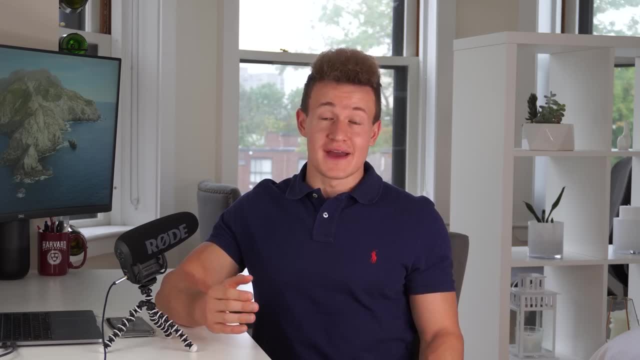 Before I dive into Feynman's problem-solving strategy, I want to show you why having great problem-solving skills is probably the most useful skill you can acquire in your entire career. It goes way beyond just solving problems. it goes way beyond just solving problems. it goes way beyond. 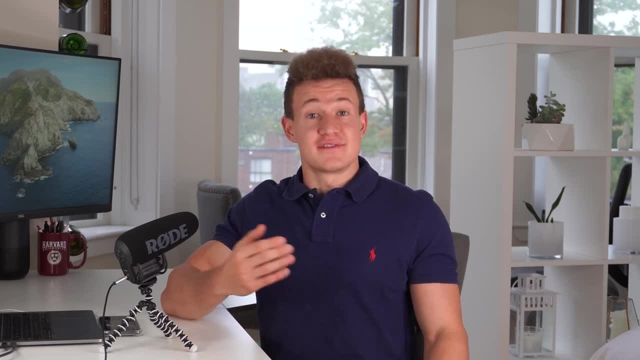 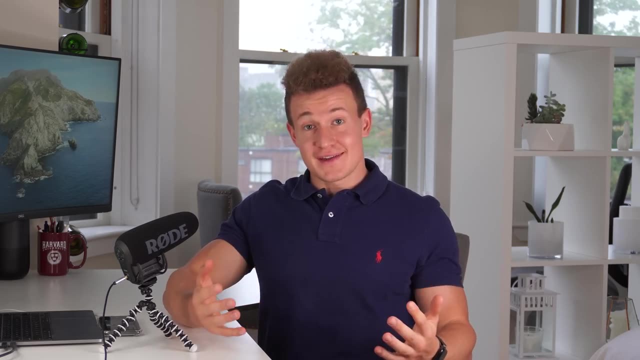 just solving math and physics problems. The reason why some entrepreneurs and CEOs end up making billions of dollars is because they managed to solve difficult problems which others were unable to solve. So you gotta ask yourself: do you want to get paid just for the hours you invest like a 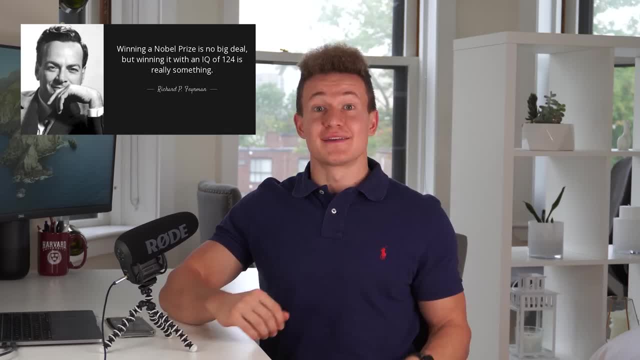 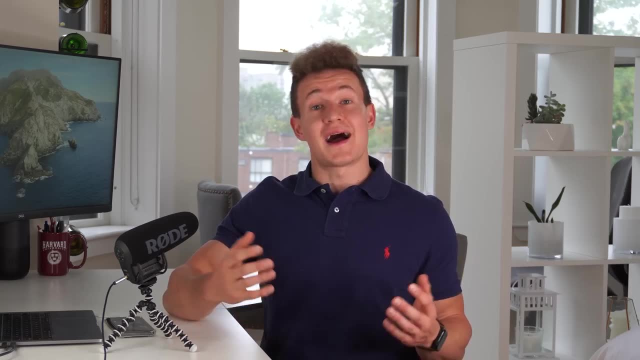 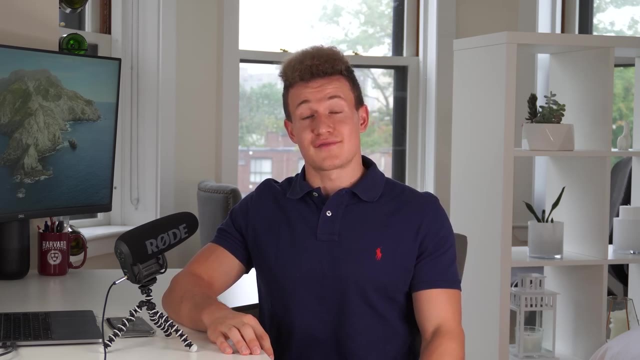 5% of the world population is actually more intelligent than him. So if Feynman could revolutionize physics with an IQ of 124 just by using clever problem-solving strategies, you can definitely do so much in your life, no matter what your IQ is. 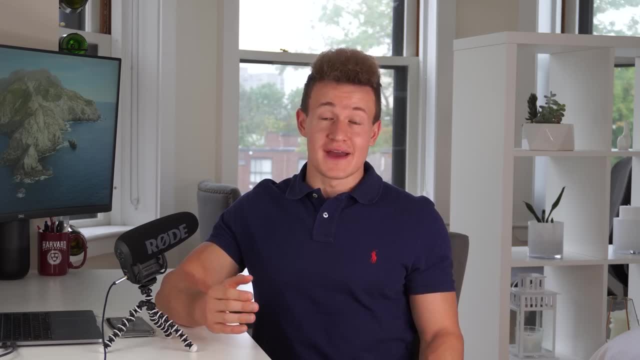 Before I dive into Feynman's problem-solving strategy, I want to show you why having great problem-solving skills is probably the most useful skill you can acquire in your entire career. It goes way beyond just solving problems. it goes way beyond just solving problems. it goes way beyond. 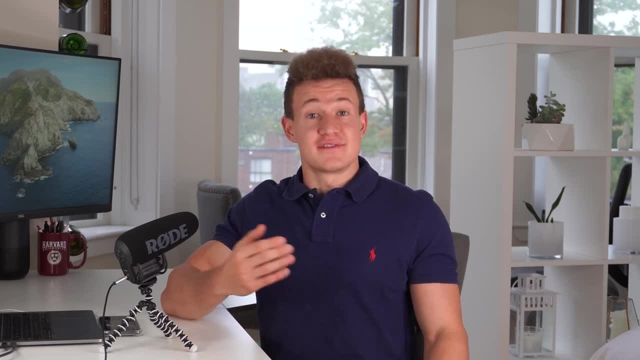 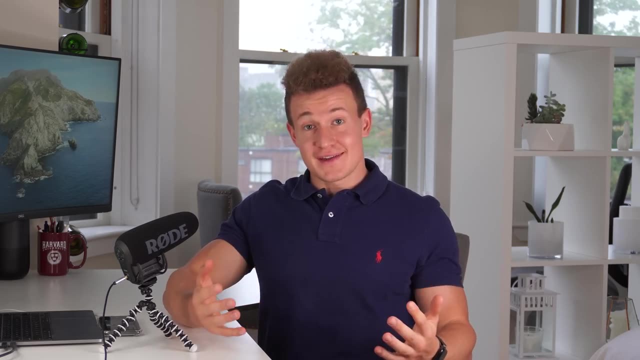 just solving math and physics problems. The reason why some entrepreneurs and CEOs end up making billions of dollars is because they managed to solve difficult problems which others were unable to solve. So you gotta ask yourself: do you want to get paid just for the hours you invest like a 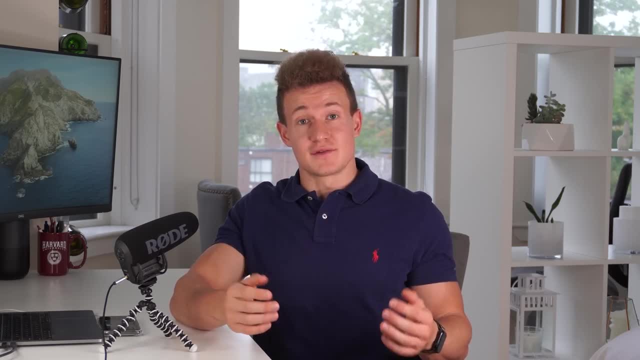 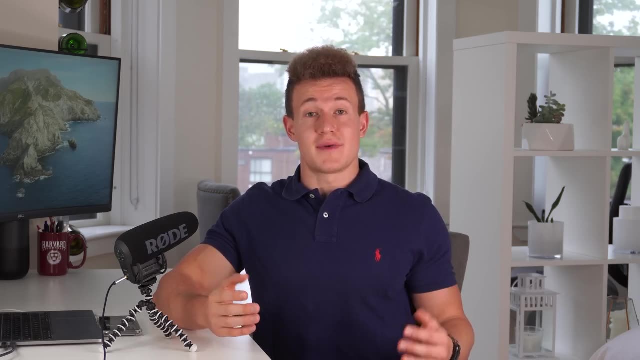 factory worker or do you want to get paid for your unique ability to solve difficult problems? A factory worker can only make linear contributions, so if he does a twice as good job, he might double the revenue for his company. therefore he might get a twice as large salary. But problem solvers- 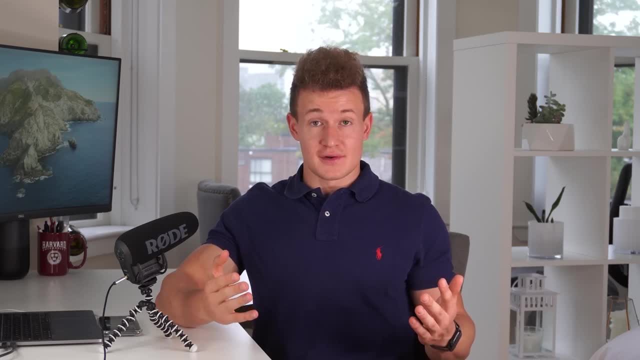 can make exponential contributions. so if you become twice as good at solving problems, you might significantly boost your company's revenue, putting almost no upper-bond on your salary. Therefore, if you want to become successful in your career, you should become a great problem. 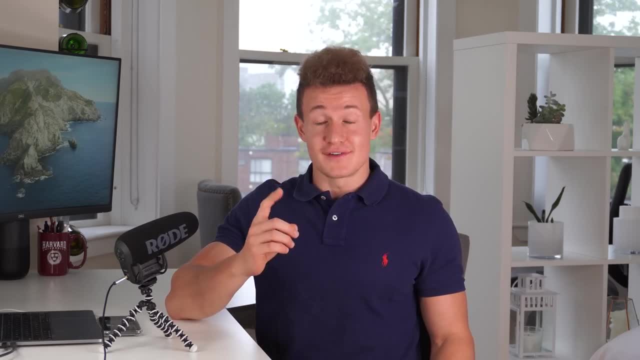 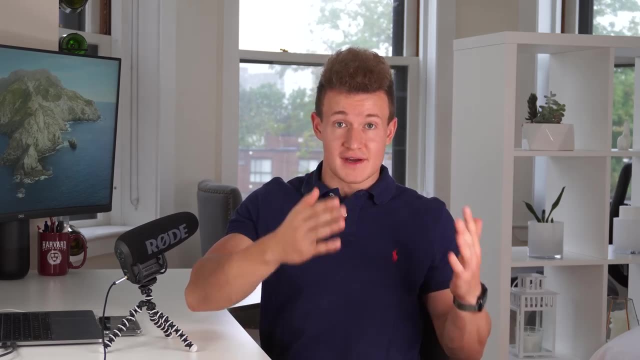 solver. Let's have a look at a problem that I made up so we can solve it using the Feynman strategy. It may be a bit too easy or too hard for you, depending on your math skills, but try to focus on the solving strategy rather than on the problem itself. A drug test is 90% sensitive and 80%. 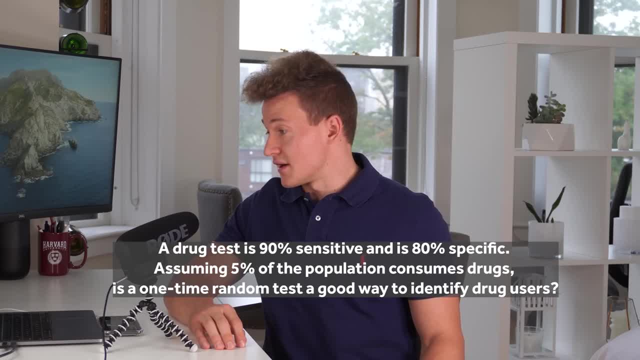 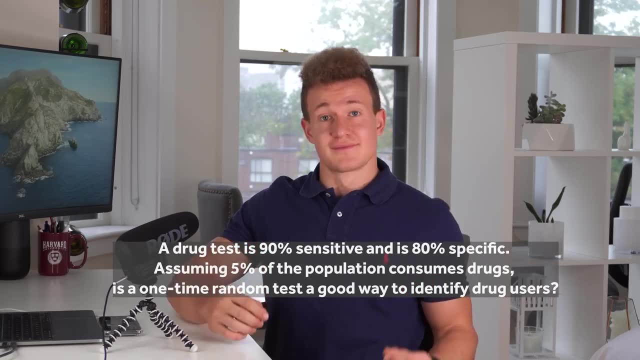 specific. Assuming 5% of the total population consumes drugs, is a one-time random test a good way to identify drug users? Feynman's problem-solving strategy works roughly as follows. Step number one is write down the problem that you want to solve, Don't just. 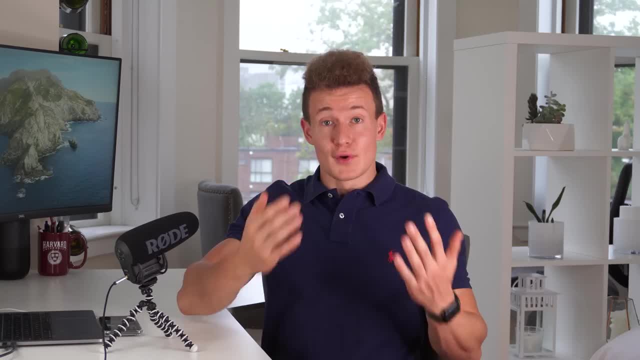 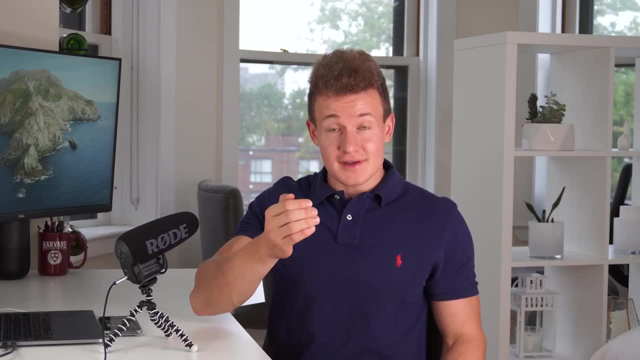 copy it from the textbook, but try to rewrite it in a way that you can fully understand it, and then try thinking about what solution you're actually looking for. For me, during physics and math competition, that meant pulling out key information, converting to appropriate 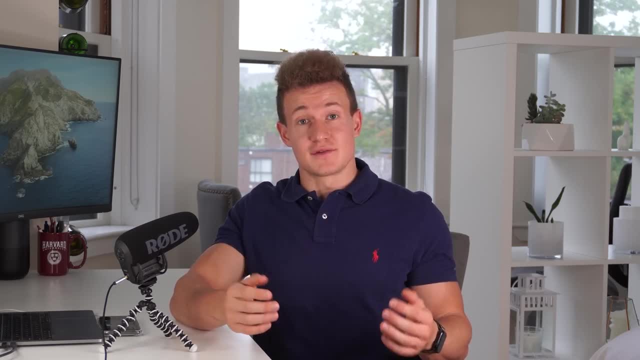 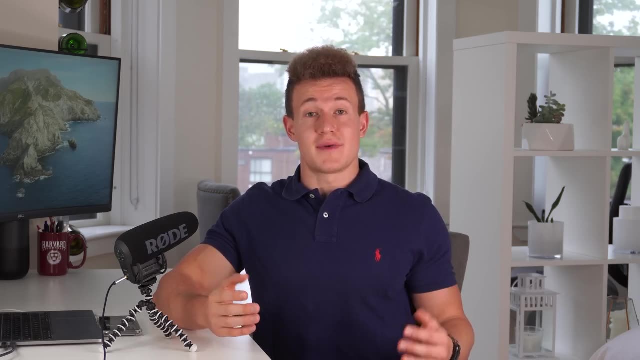 factory worker or do you want to get paid for your unique ability to solve difficult problems? A factory worker can only make linear contributions, so if he does a twice as good job, he might double the revenue for his company and therefore he might get a twice as large salary. But problem-solvers 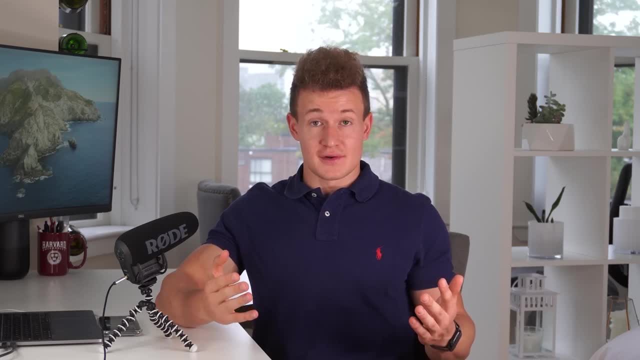 can make exponential contributions. so if you become twice as good at solving problems, you might significantly boost your company's revenue, putting almost no upper bound on your salary. Therefore, if you want to become successful in your career, you should become a great problem. 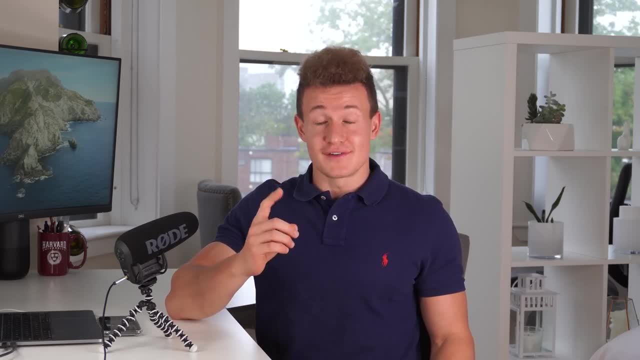 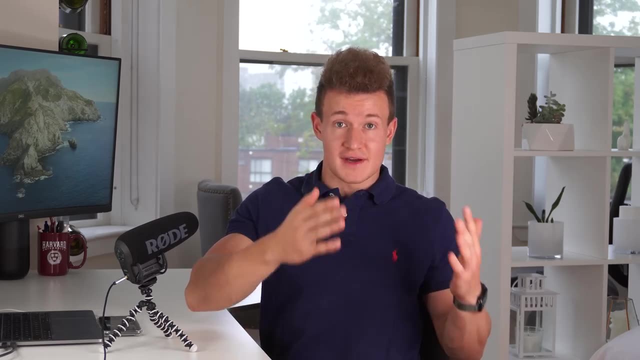 solver. Let's have a look at a problem that I made up so we can solve it using the Feynman strategy. It may be a bit too easy or too hard for you, depending on your math skills, but try to focus on the solving strategy rather than on the problem itself. A drug test is 90% sensitive and 80% specific. 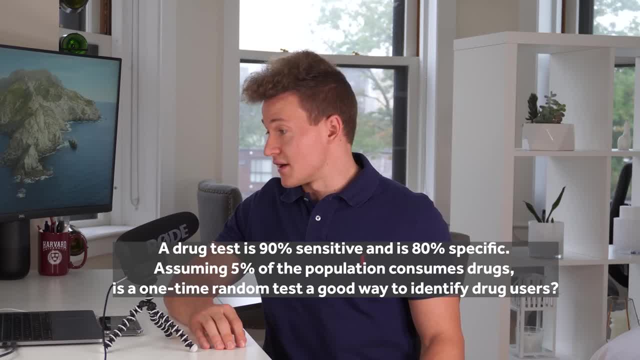 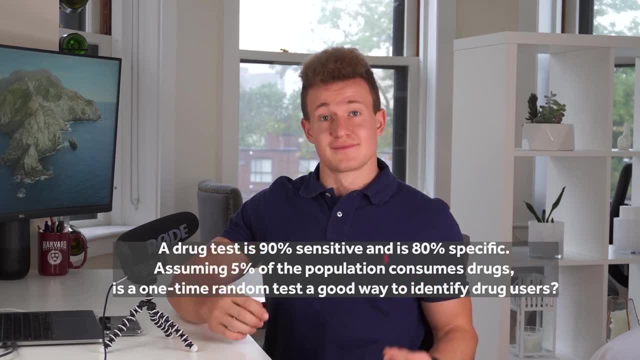 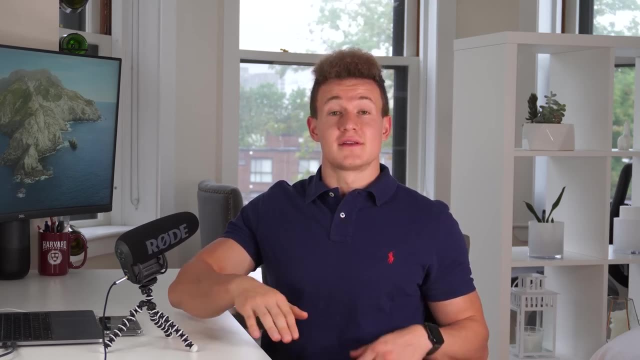 Assuming 5% of the total population consumes drugs, is a one-time random test a good way to identify drug users? Feynman's problem-solving strategy works roughly as follows. Step number one is write down the problem that you want to solve. Don't just copy it from the textbook, but try to rewrite it in a way that you can fully understand it and then try. 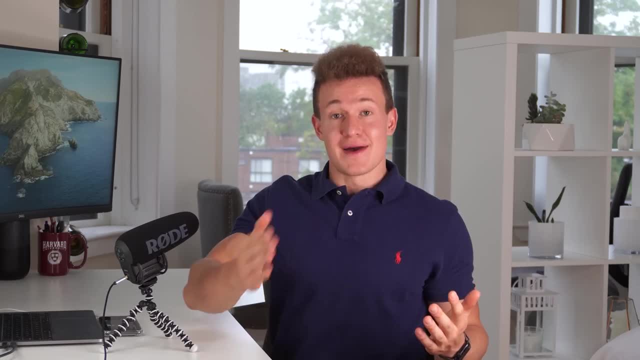 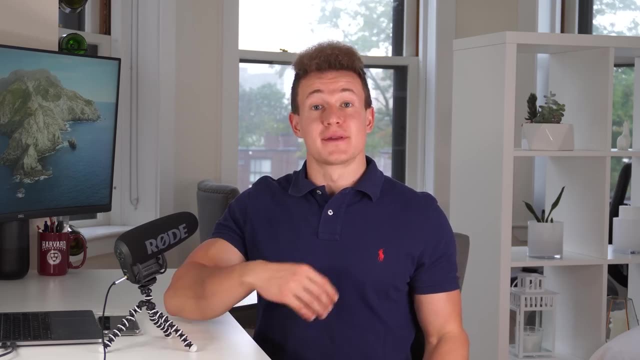 thinking about what solution you're actually looking for. For me, during physics and math competition, that meant pulling out key information, converting to appropriate units and defining key terminology. Don't feel embarrassed to spend a lot of time analyzing all of the terminology and understanding every single word in the problem. 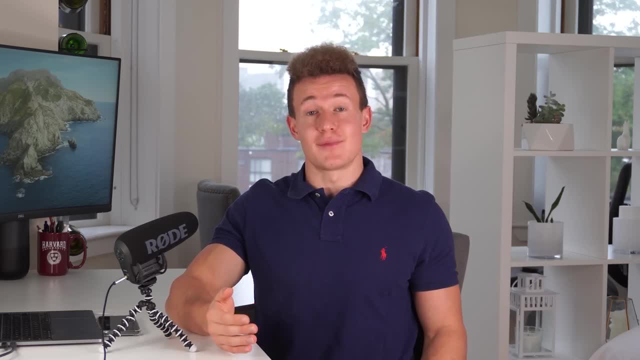 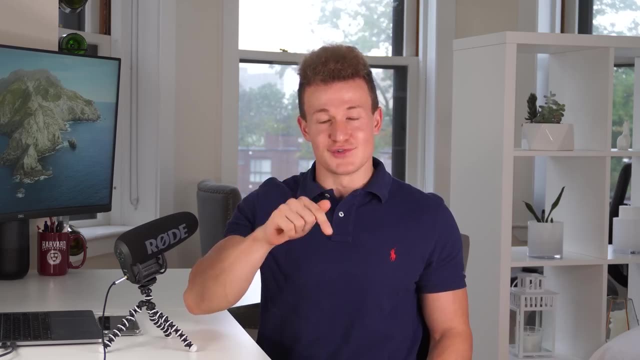 Understanding the problem can sometimes be the main step in solving the problem. So once you're confident that they understood everything, the solution might just be obvious. And if it is not obvious, then just move on to step number two. So let's apply step number one to our concrete problem. First of all. 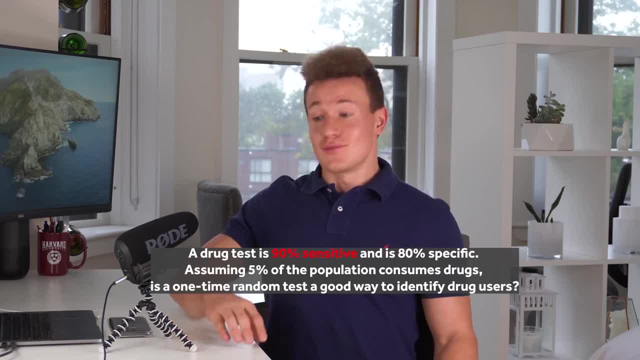 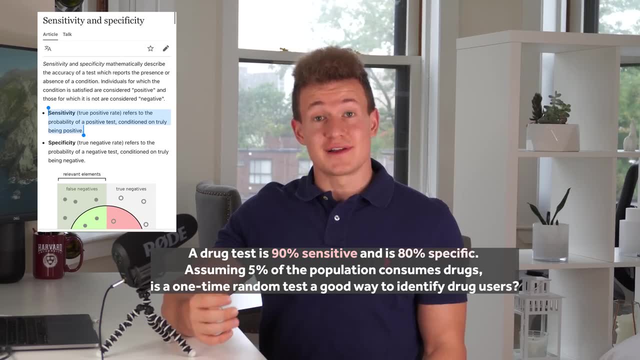 what does it mean for a drug test to be 90% sensitive? To be honest, I wasn't sure, so I had to look it up. on Wikipedia, It means that a true positive rate is 90%. Next, what does 80% specific mean? According to Wikipedia, it means that for 100 people who do not use drugs, 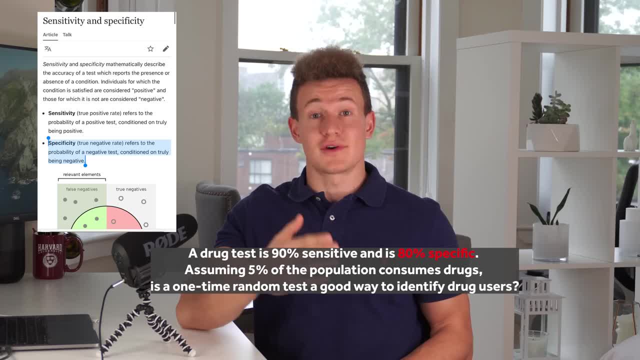 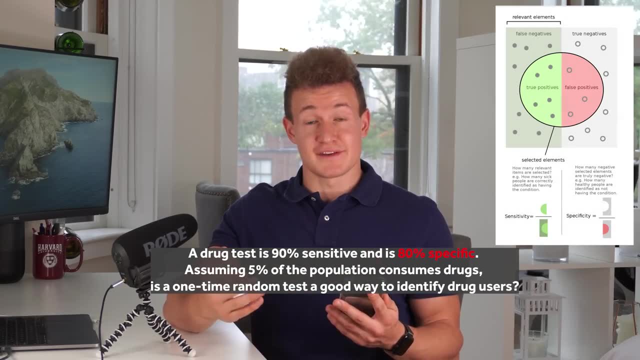 you will have 80% correctly negative results and 20% falsely positive results. If you still struggle to understand this, don't worry. just have a look at Wikipedia and the visualization will explain everything. 5% of the population consuming drugs should be pretty clear. 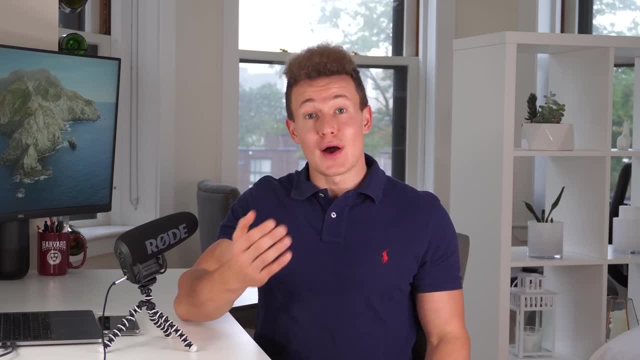 units and defining key terminology. Don't feel embarrassed to spend a lot of time analyzing all of the terminology and understanding every single word in the problem. Understanding the problem can sometimes be the main step in solving the problem. So once you're confident that you understood everything, the solution. 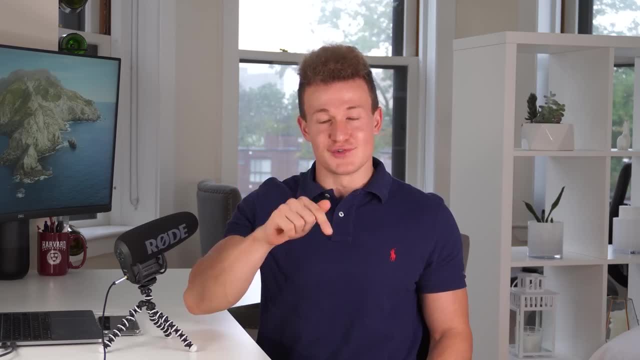 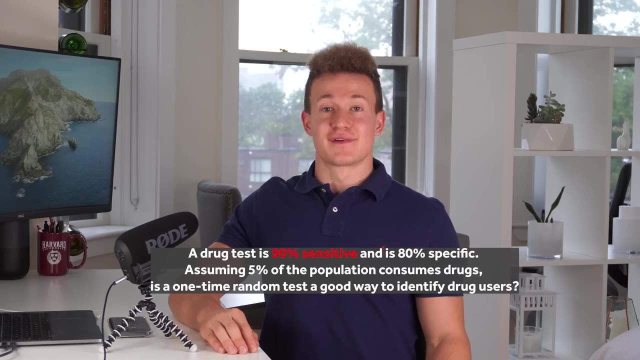 might just be obvious. And if it is not obvious, then just move on to step number two. So let's apply step number one to our concrete problem. First of all, what does it mean for a drug test to be 90% sensitive? To be honest, I wasn't sure, so I had to look it up on Wikipedia. 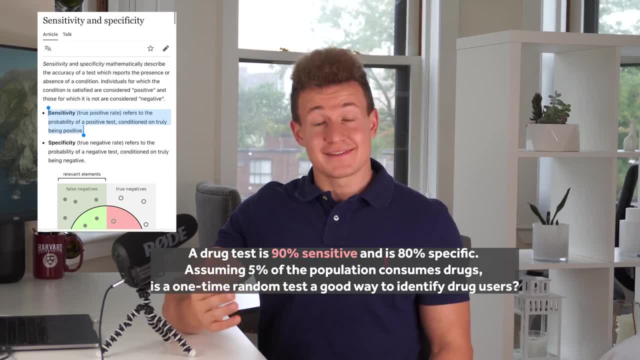 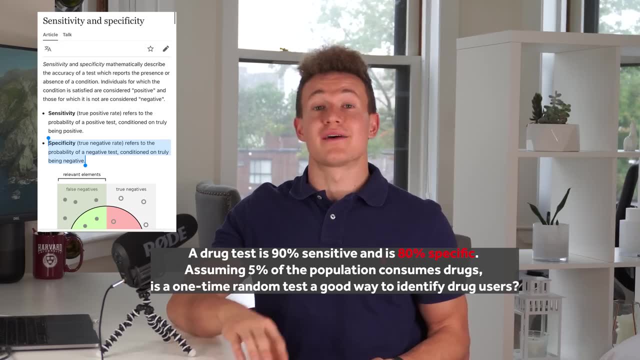 It means that the true positive rate is 90%. What does 80% specific mean? According to Wikipedia, it means that for 100 people who do not use drugs, you will have 80% correctly negative results and 20% falsely positive. 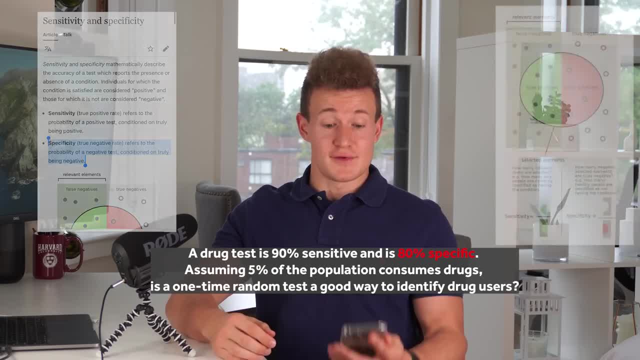 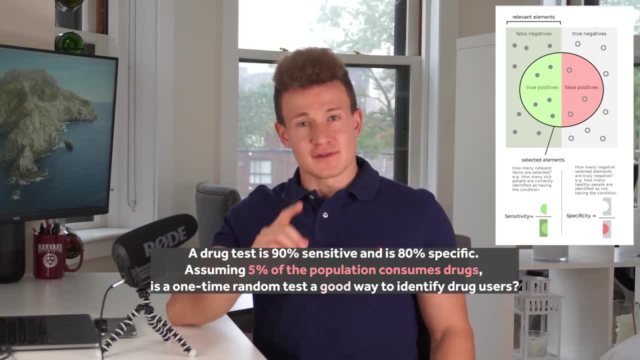 results. If you still struggle to understand this, don't worry, just have a look at Wikipedia and the visualization will explain everything. 5% of the population consuming drugs should be pretty clear. But what does good mean in this context? To understand this, let us think. 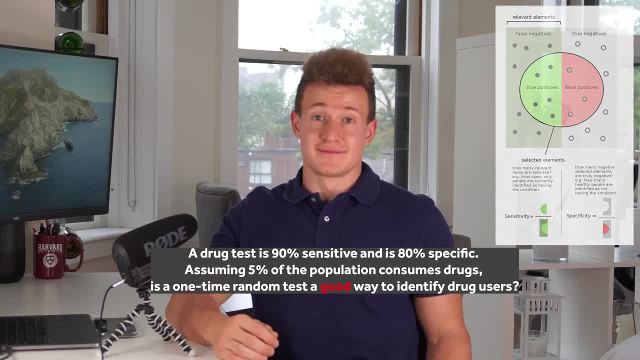 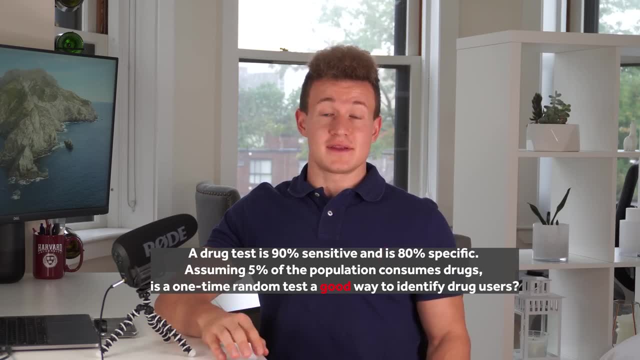 about. what would it mean for a one-time random drug test to be bad? Bad would probably mean that somebody who does not consume drugs gets randomly tested and the test ends up being positive, meaning that he gets falsely accused of using drugs even though he doesn't. So the word good in. 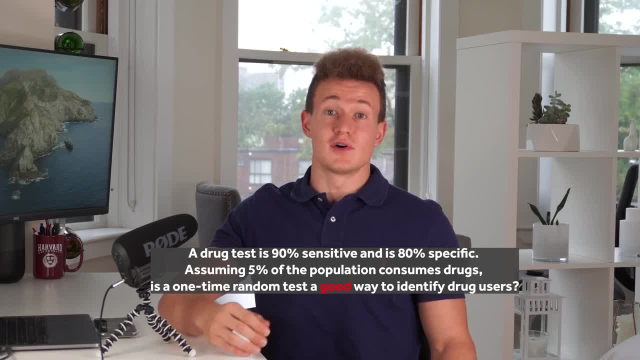 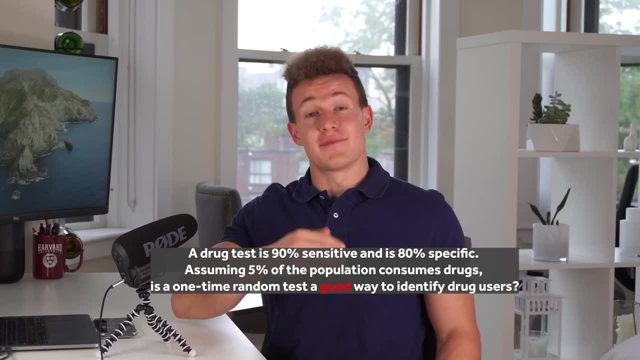 this context would mean that people rarely get accused of using drugs, even though they don't Put in mathematical terms. a test being very good means that the probability of someone actually using drugs, given that the test came back positive, is very high or close. 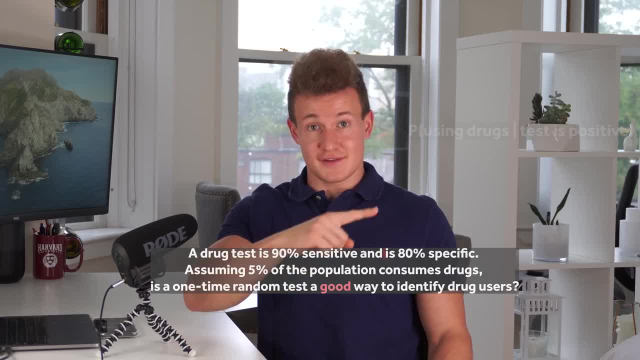 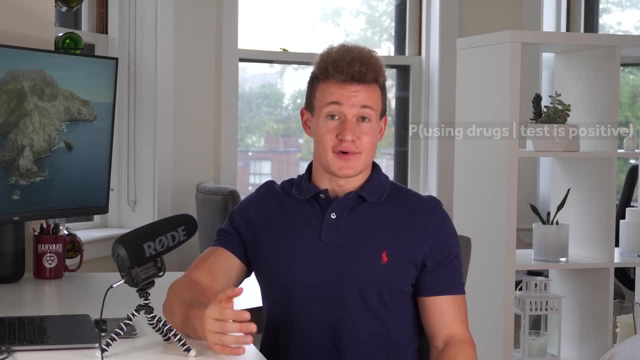 to 1.. So if we want to solve the problem, we have to calculate this quantity and check if it is close to 1.. This was step number one. Rather than just staring at a problem and thinking about it forever, we already did. 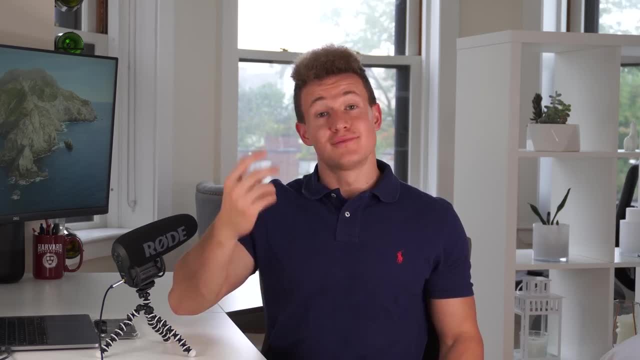 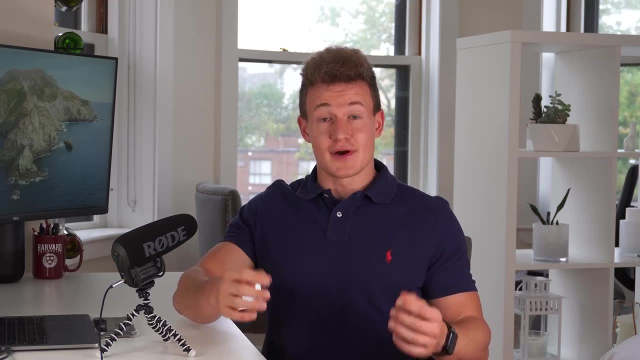 50% of the work by just analyzing it carefully. Step number two, according to Feynman, is: think really hard and try to break up the problem into smaller sub-problems that you are able to solve. Feynman's thinking process went way beyond just staring at a problem or a blank wall. 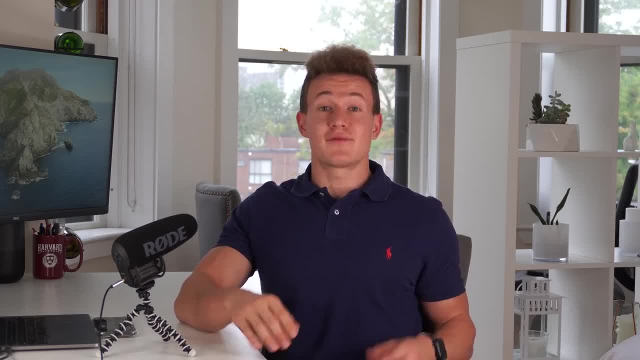 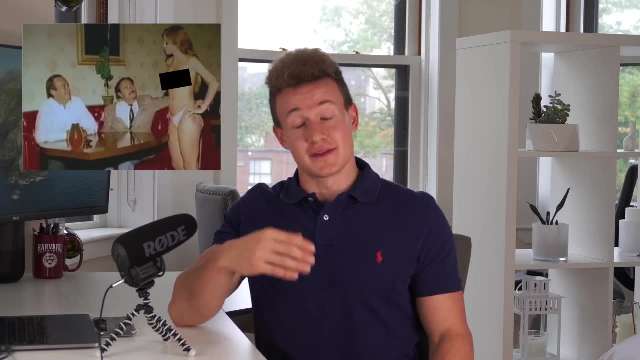 He would walk around, socialize, talk to his friends and colleagues and explain everything he knew about the problems to them. Feynman was even known for being a regular guest at a local strip club close to Caltech, where he worked after completing the Manhattan Project. 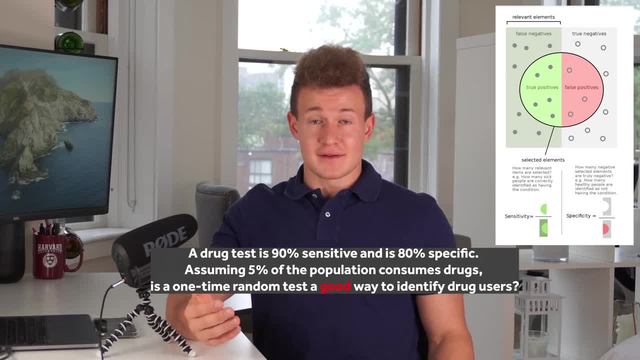 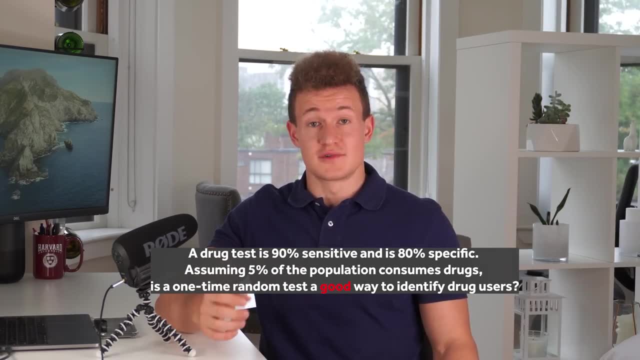 But what does good mean in this context? To understand this, let us think about what would it mean for a one-time random drug test to be bad. Bad would probably mean that somebody who does not consume drugs gets randomly tested and the test ends up being positive. 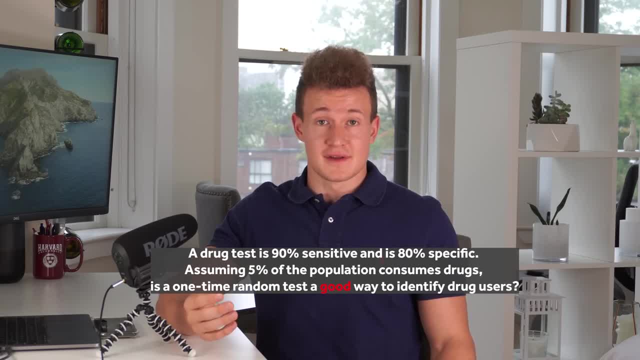 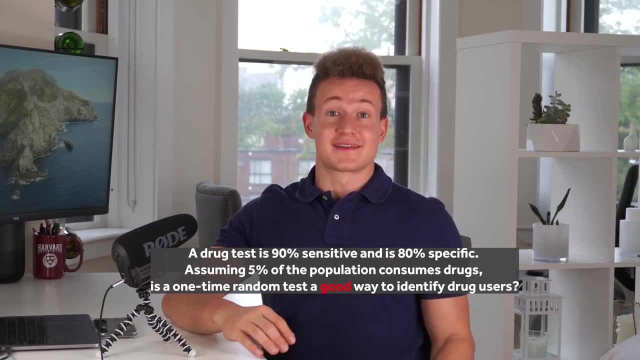 meaning that he gets falsely accused of using drugs even though he doesn't. So the word good in this context would mean that people rarely get accused of using drugs, even though they don't Put in mathematical terms. the test being very good means that the probability of someone actually using drugs 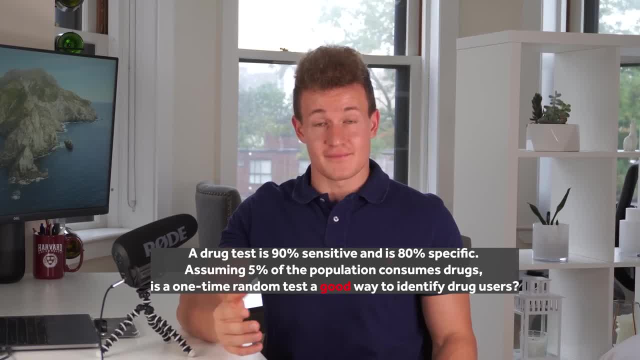 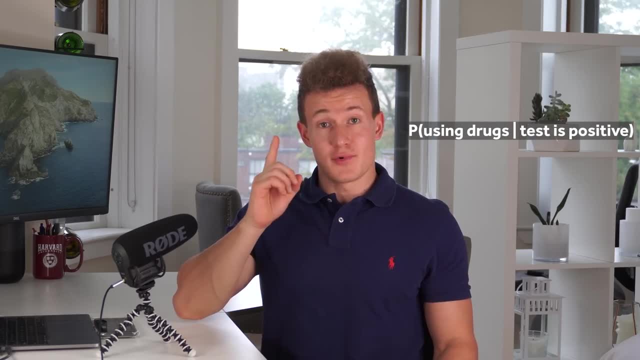 given that the test came back positive, is very high or close to one. So if you want to solve the problem, we have to calculate this quantity and check if it is close to one. This was step number one, Instead of just staring at the problem and thinking about it forever. 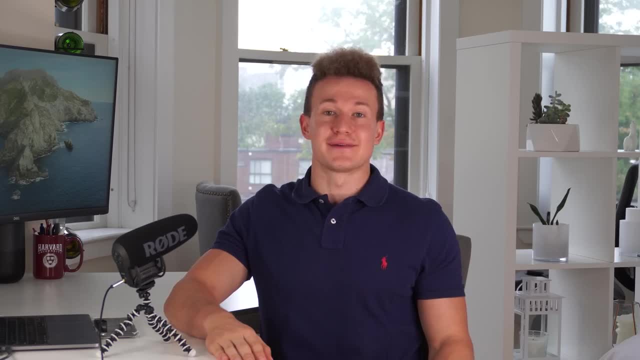 we already did 50% of the work by just analyzing it carefully. Step number two, according to Feynman, is: think really hard and try to break up the problem into smaller sub-problems that you're able to solve. Feynman's thinking process went way beyond just staring at a problem or a blank wall. 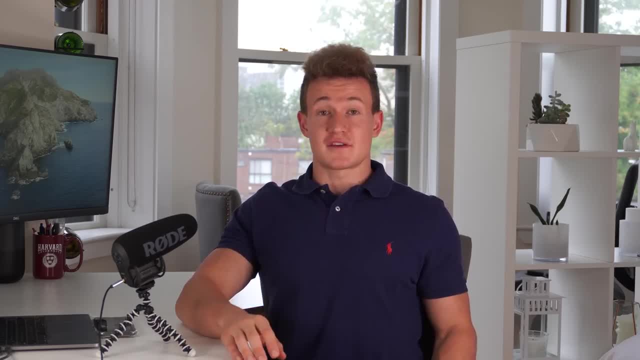 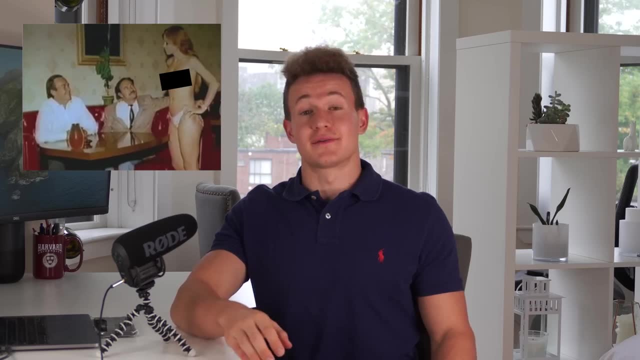 He would walk around, socialize, talk to his friends and colleagues and explain everything he knew about the problems with them. Feynman was even known for being a regular guest at a local strip club close to Caltech, where he worked after completing the Manhattan Project. 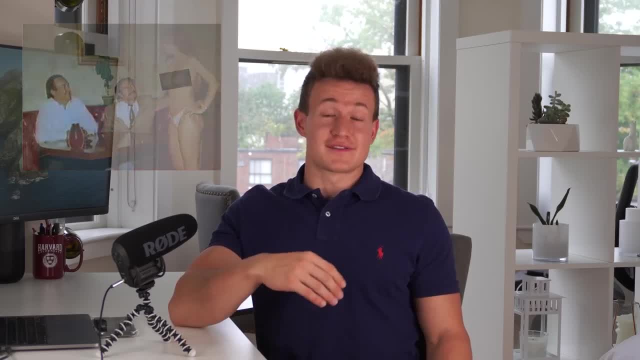 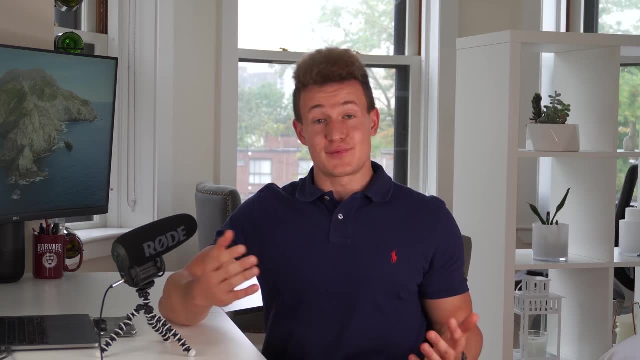 and he would go there probably five times per week, make drawings of naked girls, and then he would also work on physics problems there. While many researchers talked to each other about their scientific research and therefore make a lot of progress, Feynman's approach was really unique because he would talk to random strangers who had no idea about his field. 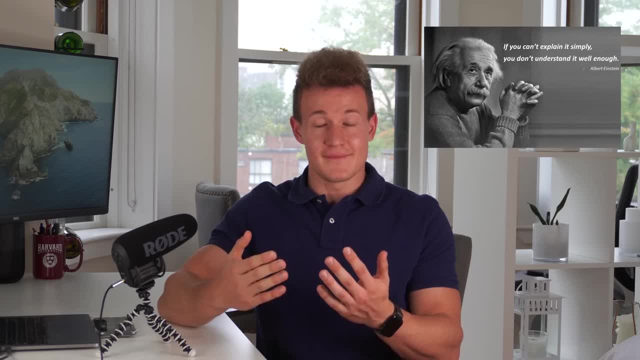 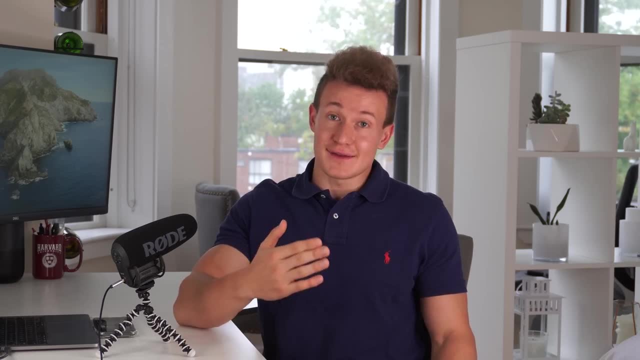 Therefore, he had to express everything in layman's terms, in a very simple way, and that helped him a lot to become a great scientist. The ideal people to talk to are curious minds who will constantly ask the why? question, like a little child. 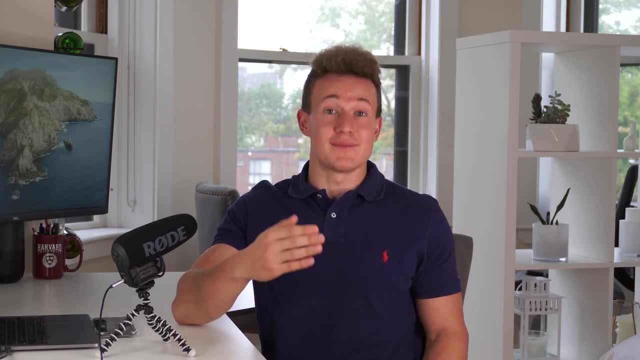 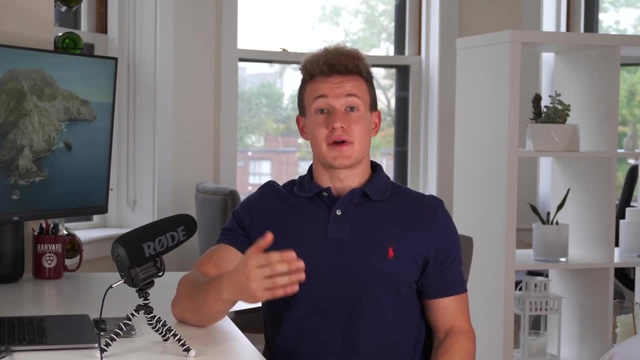 We humans are very curious beings who are constantly trying to figure out the Y band everything that we see. One could even argue that this is what makes us different from all the other animals out there. If you have to constantly explain all the problems that you're, 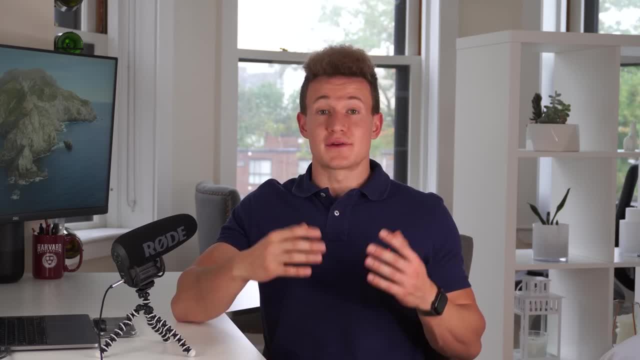 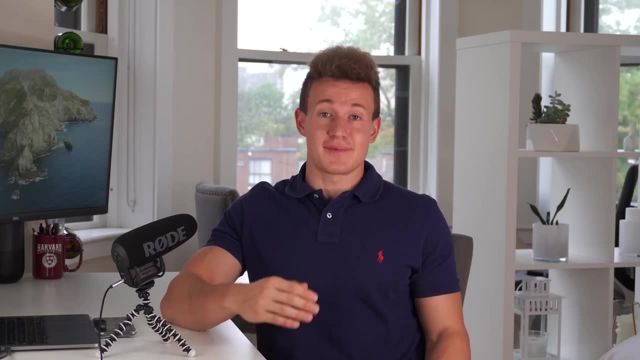 dealing with in a very simple manner. it will really help you to understand all the gaps in your knowledge and identify them very quickly. The most interesting example of a brilliant idea that Feynman came up with while explaining a simple concept is my own field of research: quantum. 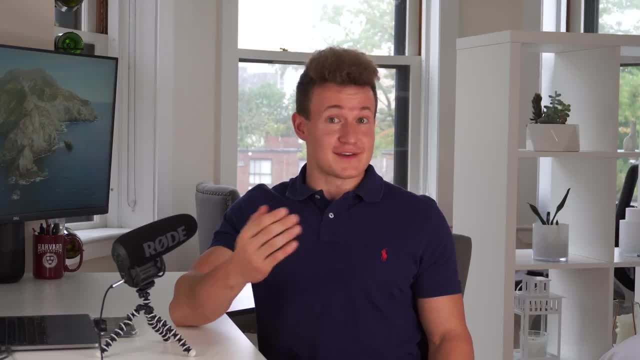 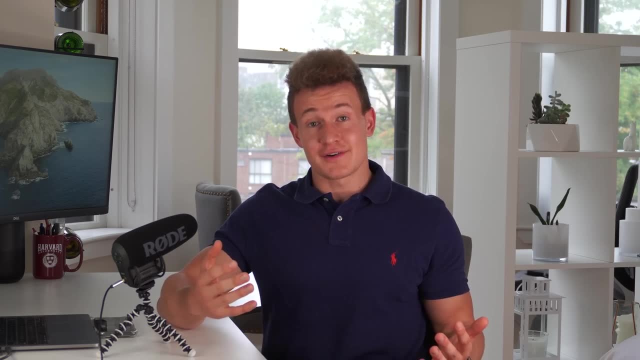 and he would go there probably five times per week, make drawings of naked girls, and then he would also work on physics problems there. While many researchers talk to each other about their scientific research and therefore make a lot of progress, Feynman's approach was really unique because he would talk to 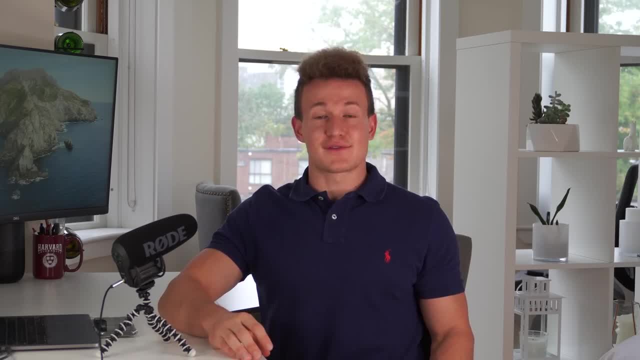 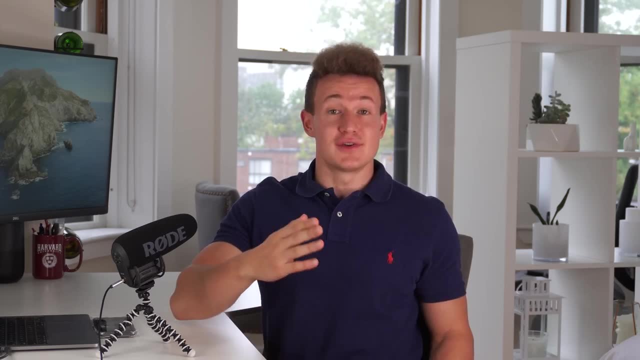 random strangers who had no idea about his field, and therefore he had to express everything in layman's terms, in a very simple way, and that helped him a lot to become a great scientist. The ideal people to talk to are curious minds who will constantly ask the why? question. 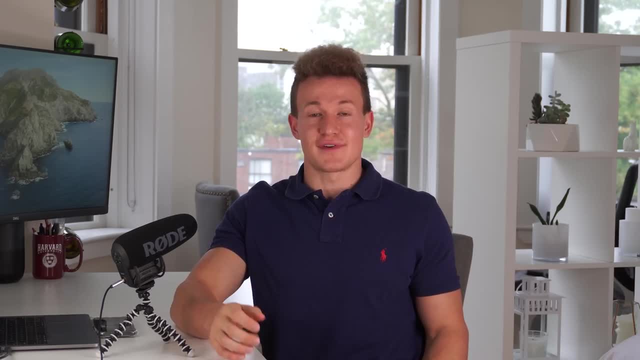 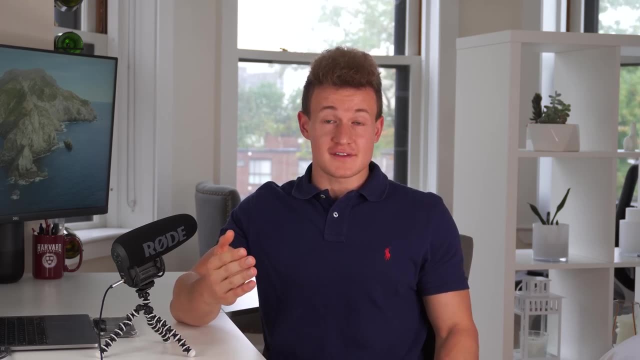 like a little child. We humans are very curious beings. we are constantly trying to figure out the why behind everything that we see. One could even argue that this is what makes us different from all the other animals out there. If you have to constantly explain all the problems that you're dealing with in a very 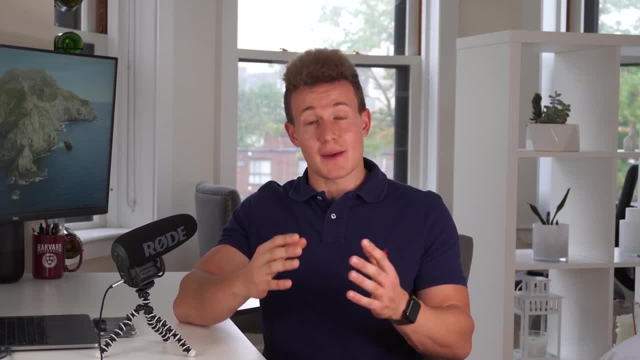 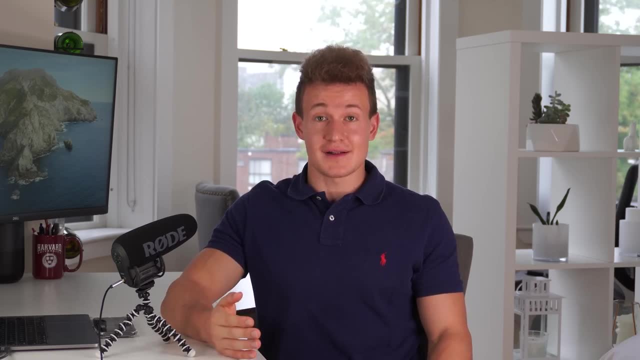 simple manner. it will really help you to understand all the gaps in your knowledge and identify them very quickly. The most interesting example of a brilliant idea that Feynman came up with while explaining a simple concept is my own field of research: quantum computing. 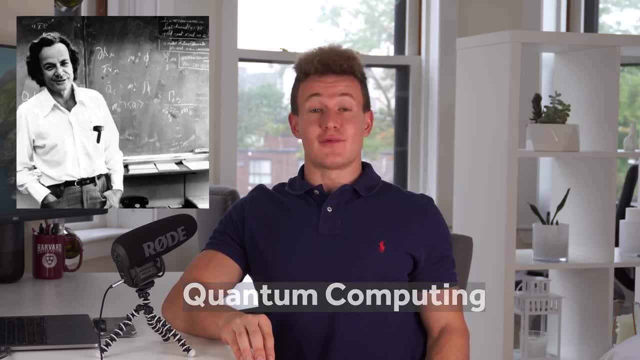 At some point during one of his physics lectures at Caltechs, he was explaining why it was so hard to simulate mathematics. He said that quantum computing is a way to simulate molecules and how interesting it would be to use quantum systems to simulate them more effectively. 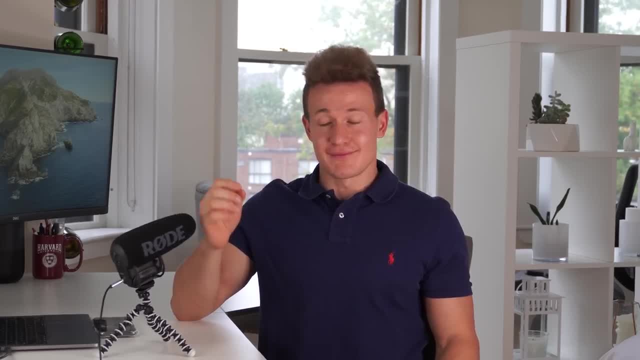 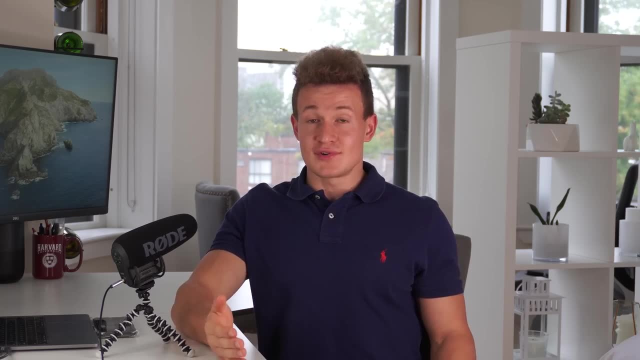 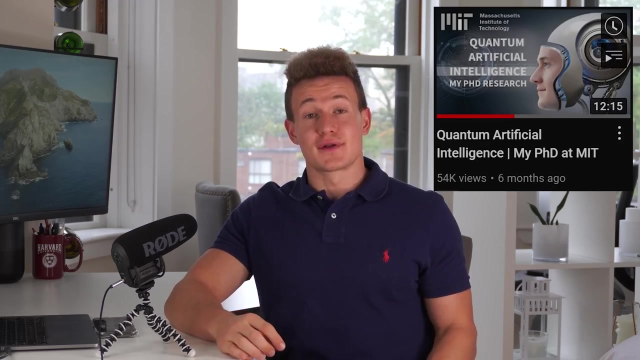 This basic idea was the spark which ignited my entire field of research. If you would like to know more about quantum computing and my PhD thesis, you can check out my video over here where I talk about all the fundamentals of quantum computing. Some of the most difficult concepts that I ever had to understand in my life were concepts 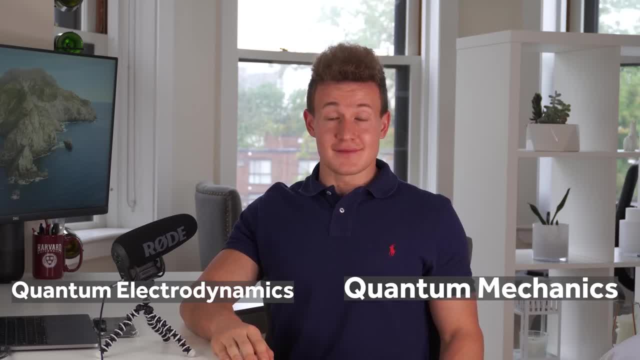 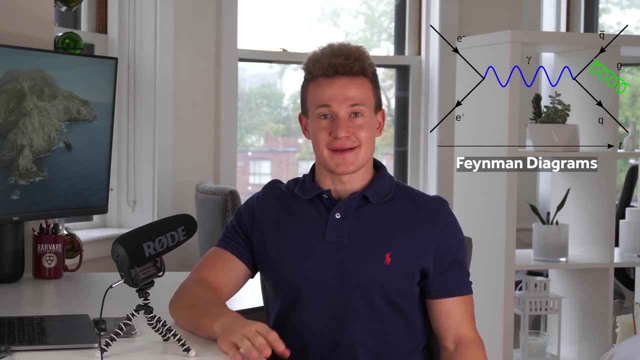 in quantum mechanics and quantum electrodynamics. Coincidentally, Many of these concepts were actually initially discovered by Richard Feynman. The most difficult exam I had in my entire life was my quantum mechanics final exam. Luckily, I found two good friends who were roughly as knowledgeable as I am, so we spent 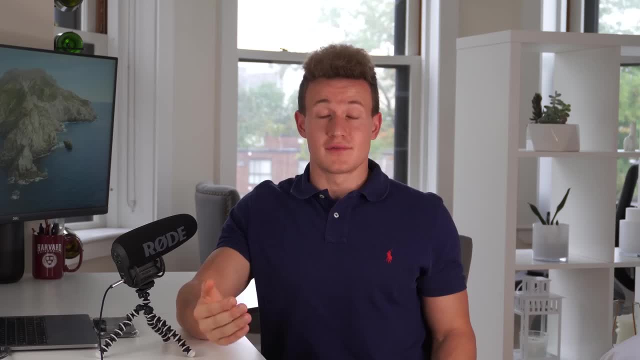 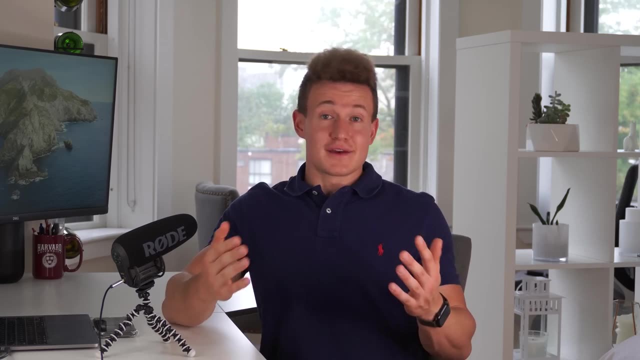 the mornings trying to understand the concepts on our own, and in the afternoon we would come together, usually without understanding much, and try to puzzle everything together until all of us would understand the difficult concepts At later points in my study. I wasn't lucky enough to find someone to study with, but 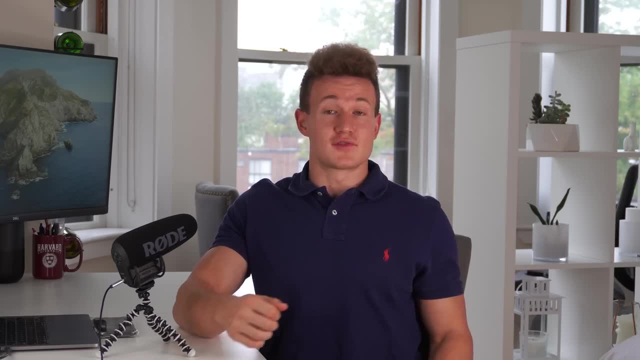 it was okay, I would just study on my own and I would try to explain all these concepts either to my dog, Milky, or to my friends. If you are a university student, you could, for example, become a teaching assistant. Just make sure that you will be actually teaching and not just spending your time grading quizzes. 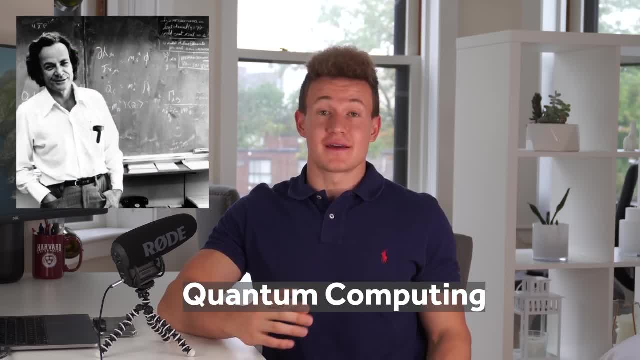 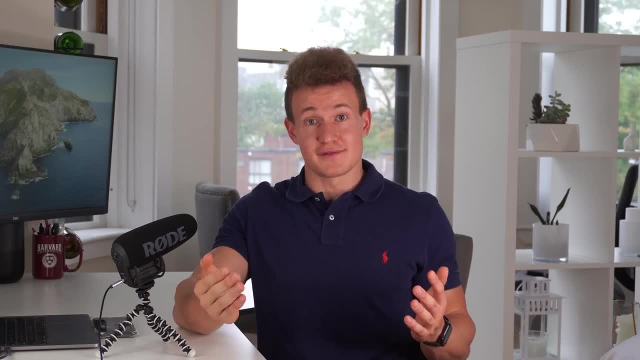 computing. At some point during one of his physics lectures at Caltechs, he was explaining why it was so hard to simulate molecules and how interesting it would be to use quantum systems to simulate them more effectively. This basic idea was the spark which ignited my entire field of quantum. 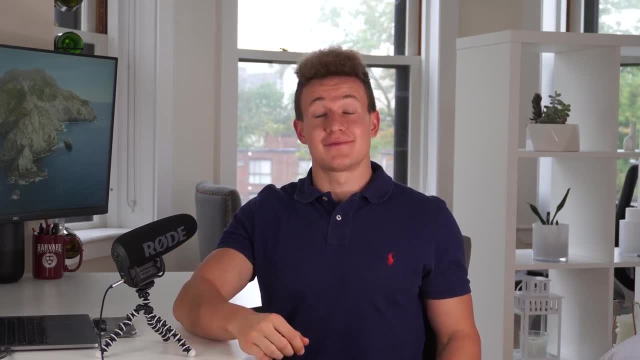 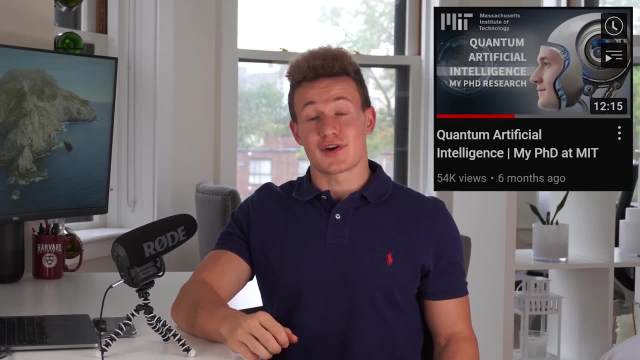 Oops, I hit the. This basic idea was the spark which ignited my entire field of research. If you would like to know more about quantum computing in my PhD thesis, you can check out my video over here where I talk about all the fundamentals of quantum computing. Some of the 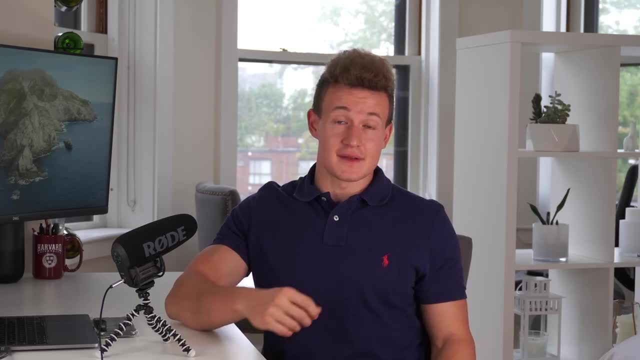 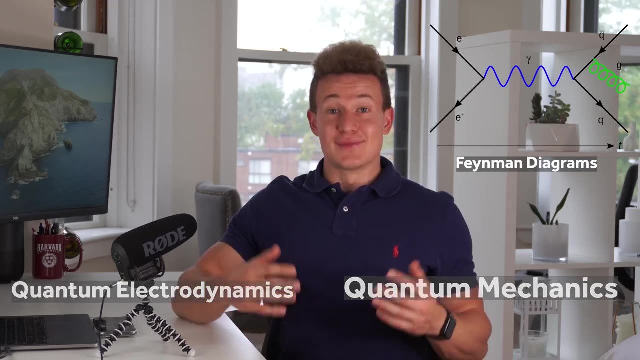 most difficult concepts that I ever had to understand in my life were concepts in quantum mechanics and quantum electrodynamics. Coincidentally, quantum mechanics is a concept that many of these concepts were actually initially discovered by Richard Feynman. The most difficult exam I had in my entire life was my quantum mechanics final exam. 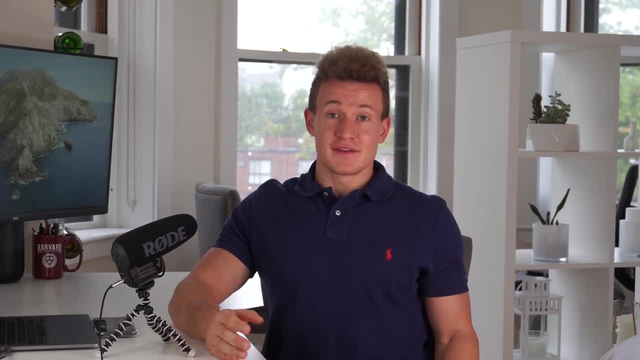 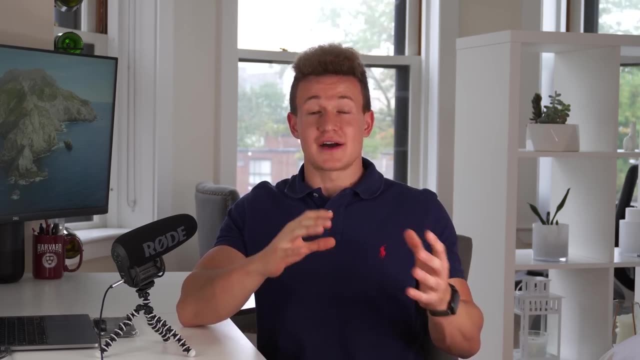 Luckily I found two good friends who were roughly as knowledgeable as I am, so we spent the mornings trying to understand the concepts on our own, and in the afternoon we would come together, usually without understanding much, and try to puzzle everything together until all of us would understand the difficult concepts At later points in my study. 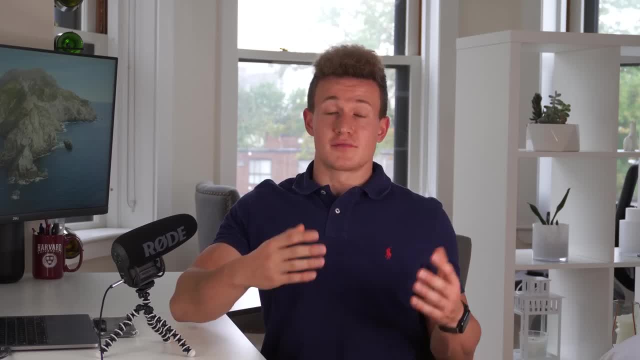 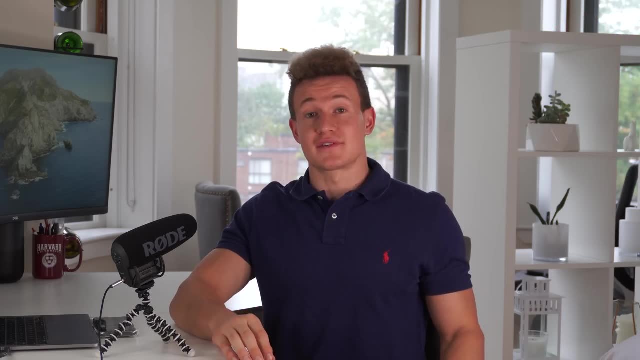 I wasn't lucky enough to find someone to study with, but it was okay. I would just study on my own and I would try to explain all these concepts either to my daughter, or to my friend, or to my dog, Milky, or maybe to some of my plants. If you are a university student, you could, for example: 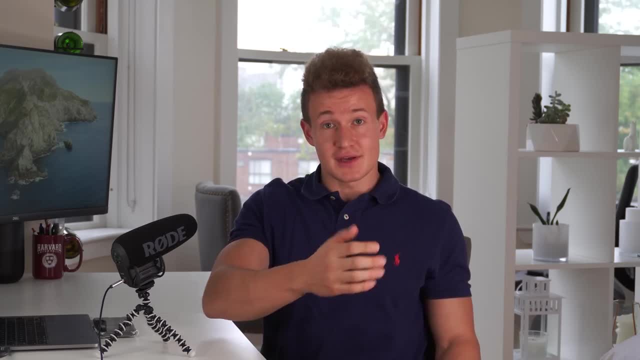 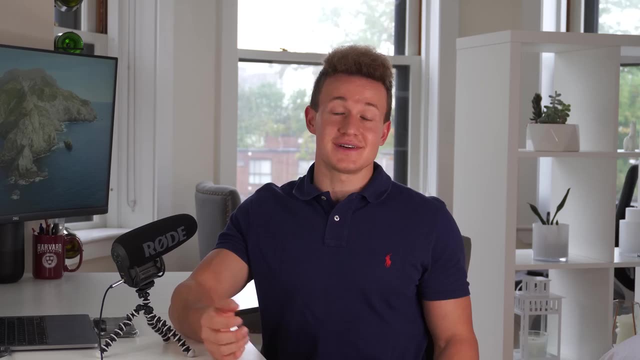 become a teaching assistant. Just make sure that you will be actually teaching and not just spending your time grading quizzes and exams. I myself volunteered to host the physics olympiad preparations in my home country, Croatia. This allowed me to rediscover physics with some of 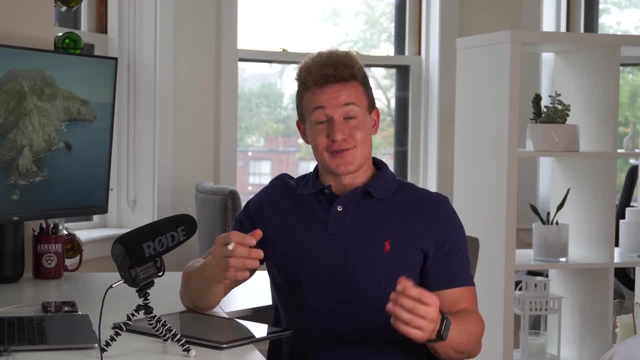 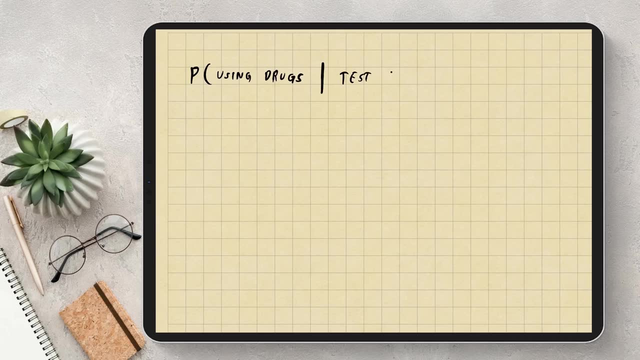 the smartest and most curious minds in the entire country. Back to our drug testing problem. We know that for a random test to be good, it means that the probability of someone actually using drugs, given that the test came back positive, needs to be somewhere close to 1.. Let's have a look at this quantity. 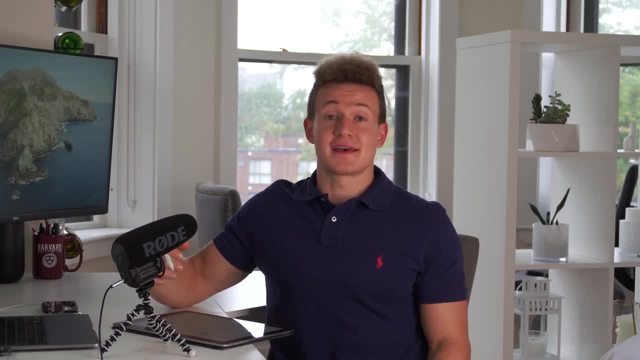 The probability of someone using drugs, given that the test came back positive. So if this doesn't really look familiar to you, this would be the point where you would start talking to friends and colleagues until somebody would eventually probably tell you that this looks. 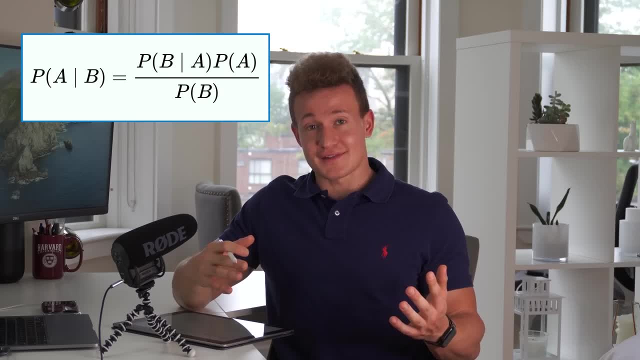 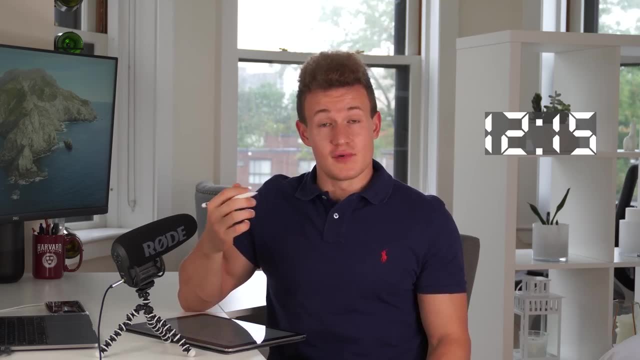 a lot like the Bayes theorem. Obviously, I can't really demonstrate that process over here, but let's just assume I got this information from someone. Feel free to skip to this timestamp for step number three or just continue watching. Solve the Problem. 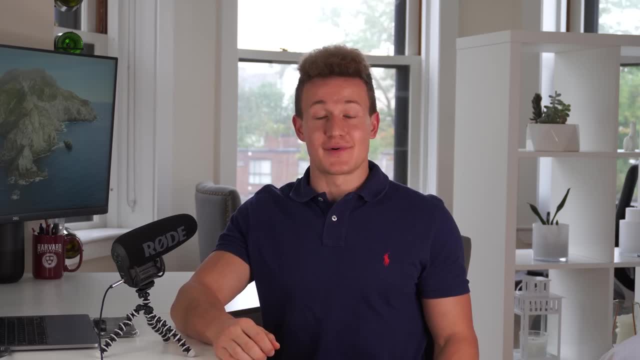 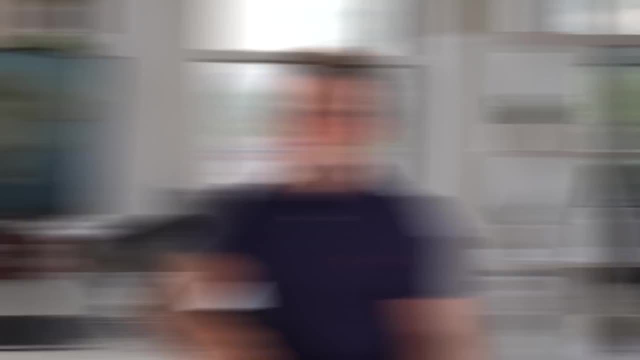 and exams. I myself volunteered to host the physics olympiad preparations in my home country, Croatia. This allowed me to rediscover physics with some of the smartest and most curious minds in the entire country. Back to our drug testing problem. We know that for a random test to be good, it means that the probability of someone actually 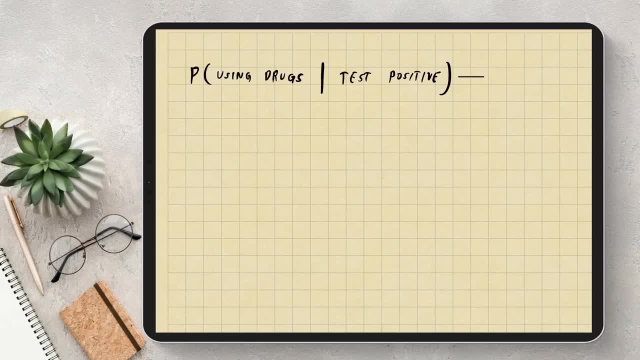 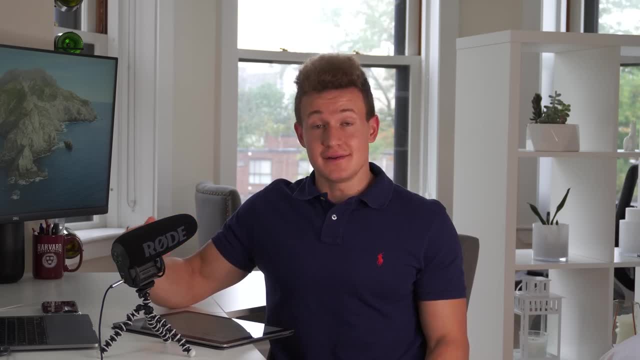 using drugs, Given that the test came back positive, Needs to be somewhere close to one. Let's have a look at this quantity: The probability of someone using drugs, given that the test came back positive. So if this doesn't really look familiar to you, this would be the point where you would 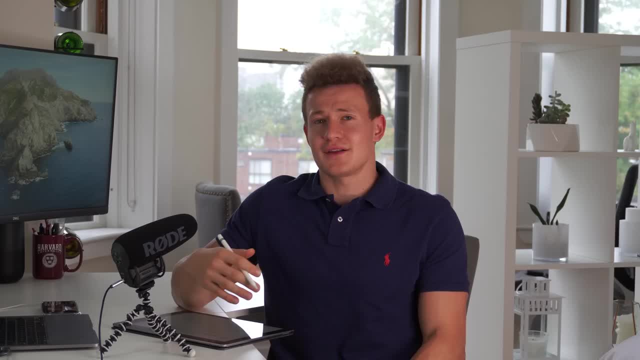 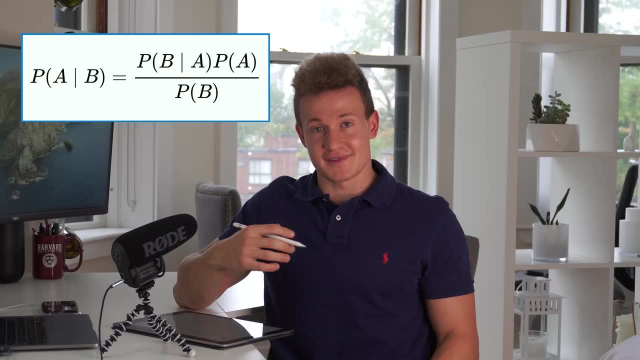 start talking to friends and colleagues until somebody would eventually probably tell you that this looks a lot like the Bayes theorem. Obviously, I can't really demonstrate that process over here, but let's just assume I got this information from someone. Feel free to skip to this timestamp for step number three or just continue watching Solve. 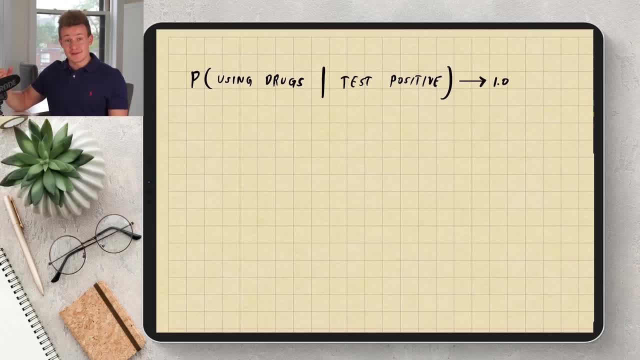 the Problem. So, first of all, I'm going to start by writing down the Bayes theorem in a way that will be very easy to analyze and then compare the two quantities. So let's get started. So far I haven't really done anything new, but now, when you look at this, you can very 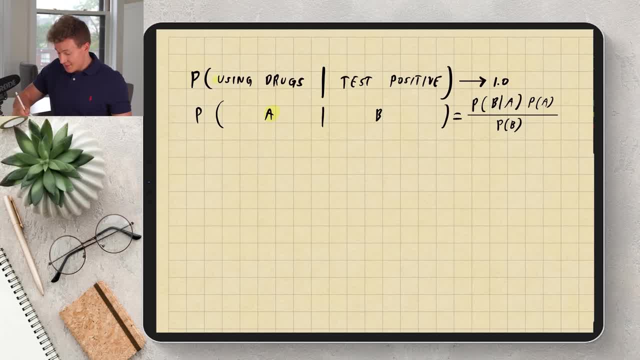 easily see in the first and second line that A is equivalent to using drugs and B is just equivalent to the test being positive. So now that we know what the quantities mean, it should be very easy to solve the rest of the problem. All right, so now that we know exactly what is what, we can just look at the Bayes formula. 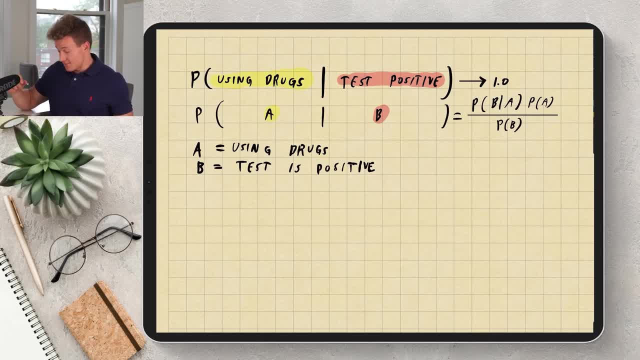 and try to figure out if we can find what the quantities on the right side are, That is, P of B given A, P of A and P of B. So first of all, let's start with P of B given A, But that is just the probability of the test being positive, given that someone is using 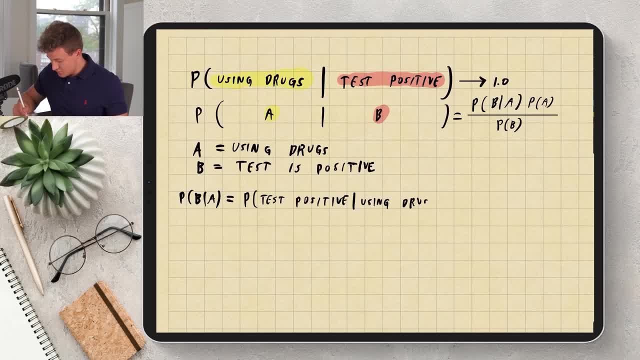 drugs. So let's start with P of B given A, But that is just the probability of the test being positive, given that someone is using drugs. So this quantity is just equal to the sensitivity, that is the true positives, which is 90% or 0.9.. 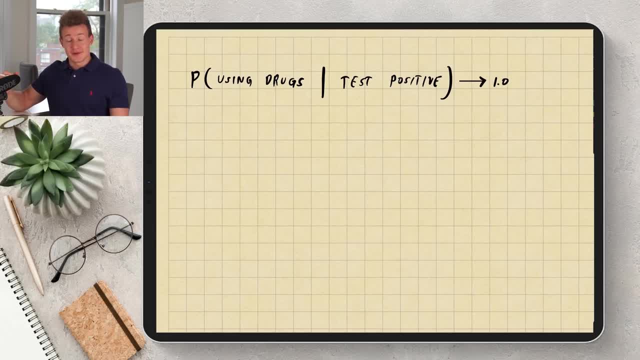 So, first of all, I'm going to show you how to solve the problem. So, first of all, I'm going to start by writing down the Bayes theorem in a way that will be very easy to analyze and then compare the two quantities. So let's get started. 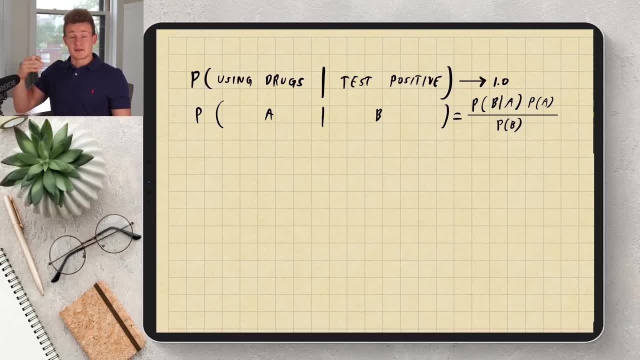 So far I haven't really done anything new, but now when you look at this, you can very easily see in the first and second line that A is equivalent to using drugs and B is just equivalent to the test being positive. So now that we know what the quantities mean, it should be very easy to solve the rest of the 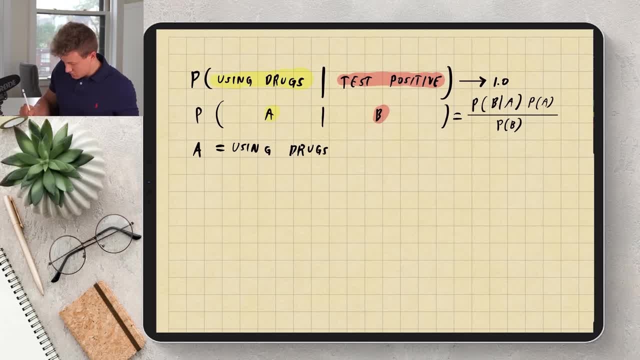 problem. All right, so now that we know exactly what is what, we can just look at the Bayes formula and try to figure out if we can find what the quantities on the right side are, That is, P of B given A, P of A and P of B. So first of all, let's start with P of B given A. 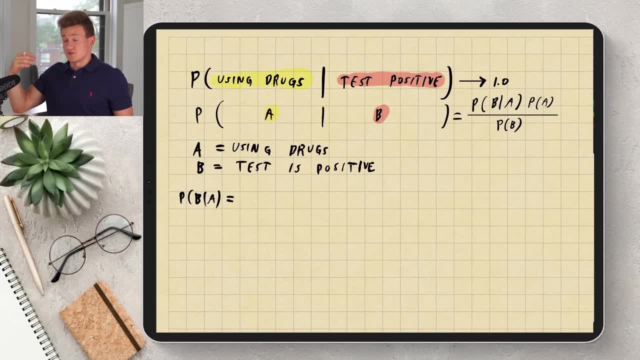 But that is just the probability of the test being positive, given that someone is using drugs. So this quantity is just equal to the sensitivity, that is the true positives, which is 90% or 0.1, 0.9.. 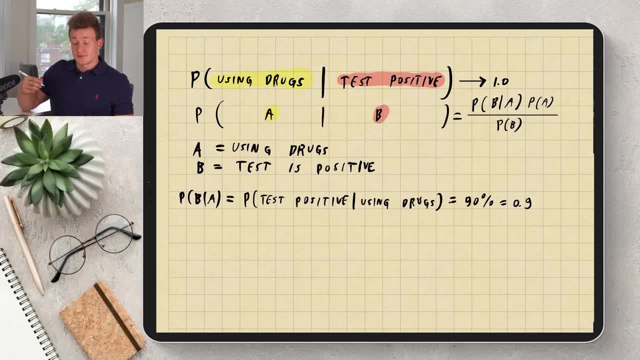 The next quantity is just P of A, which is the probability of someone using drugs. Well, we already know that number. that's just 5% of the people in total are using drugs. But the last quantity that we have to figure out is P of B. 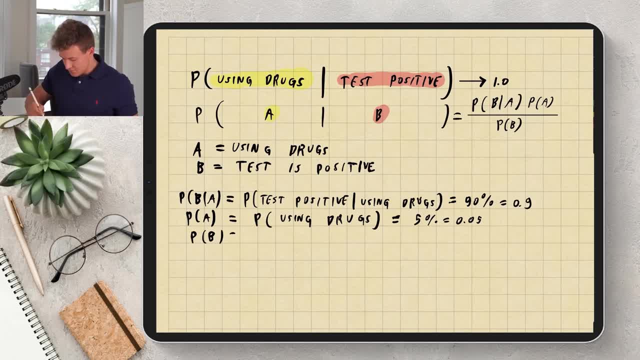 that is the probability of the test being positive. So this may actually be the most tricky part of this whole problem to figure out, because it's asking us for the probability of a randomly selected person to be positive. So if you can't really figure out what a number would be, 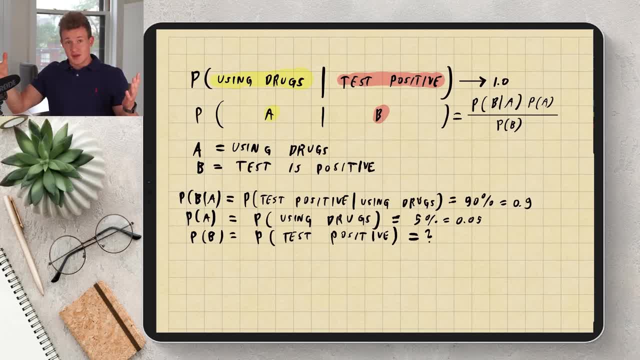 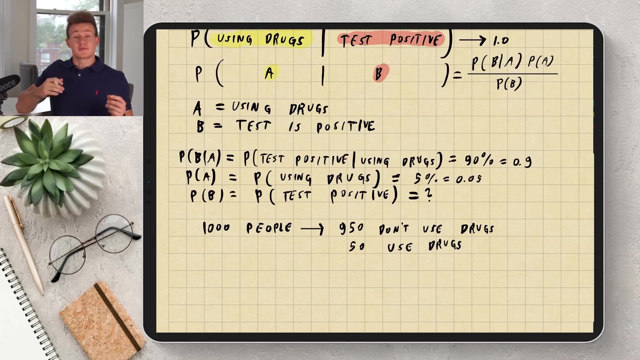 it's actually quite easy to analyze by just imagining a group of 1,000 people in total. Now, of these 1,000 people, 950 will not be using drugs and 50 will be using drugs. Now all that is really left to do is count how many of these tests are going to be positive for each of these two different groups. 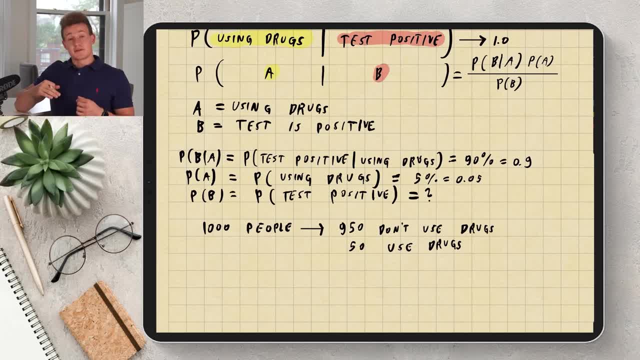 So now, instead of just looking at the 1,000 people as one group, we can just split it up into 950 people who do not use drugs- and there we know how the test behaves- and 50 people who do use drugs, and we also know how the test behaves for them. 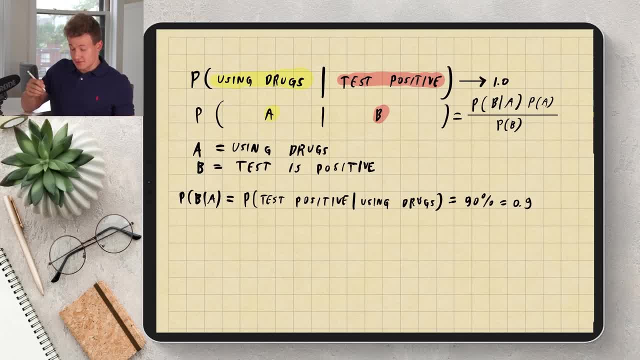 The next quantity is just P of A, which is the probability of someone using drugs. Well, we already know that number. that's just 5% of the people in total are using drugs. But the last quantity that we have to figure out is P of B, that is the probability of 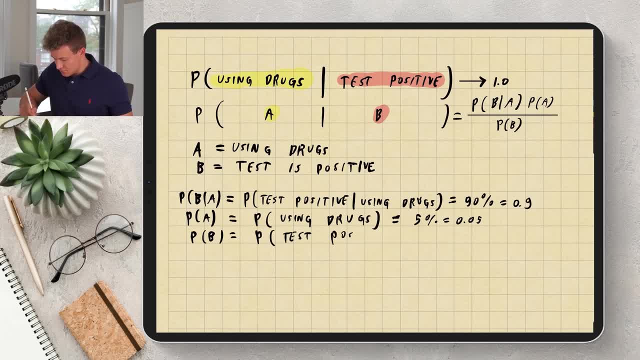 the test being positive. So this may actually be the most tricky part of this whole problem to figure out, because it's asking us for the probability of a randomly selected person to be positive. So if you can't really figure out what a number would be, it's. 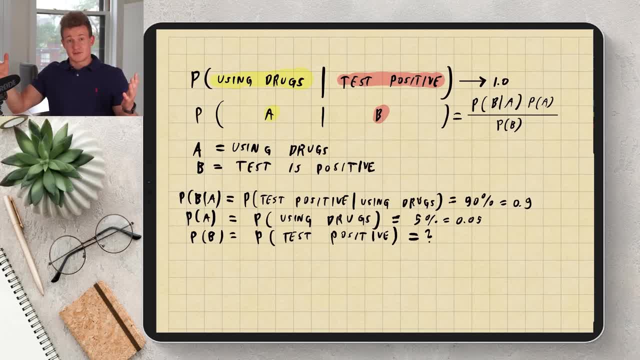 actually quite easy to analyze by just imagining a group of 1,000 people in total. Now, of these 1,000 people, 950 will not be using drugs and 50 will be using drugs. Now, all that is really left to do is count how many of these tests. 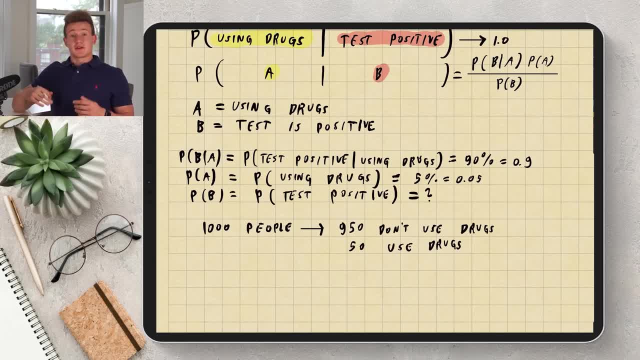 are going to be positive for each of these two different groups. So now, instead of just looking at the 1,000 people as one group, we can just split it up into 950 people who do not use drugs, and there we know how the test behaves. 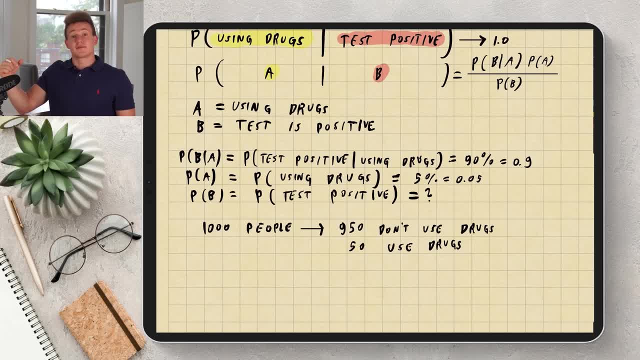 and 50 people who do use drugs, and we also know how the test behaves for them. So let's first look at the 950 people. We know that the false positive tests are going to be 20%, So we just have to multiply 20% by 950 in order to get how many false positive 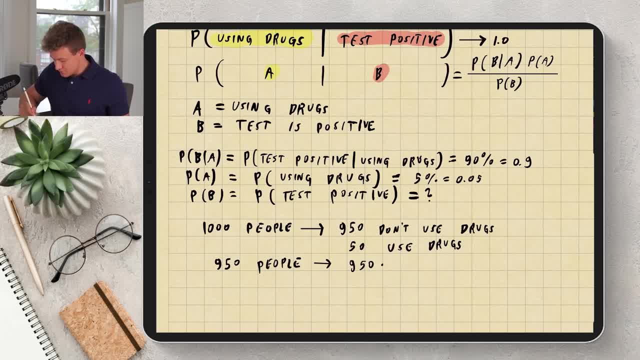 tests we're going to have. So there's a total of 190 false positive tests For the 50 people. we also know how the test behaves, Namely, we know that for 90% of the people who actually do use drugs, the test is going to trigger and it's going. 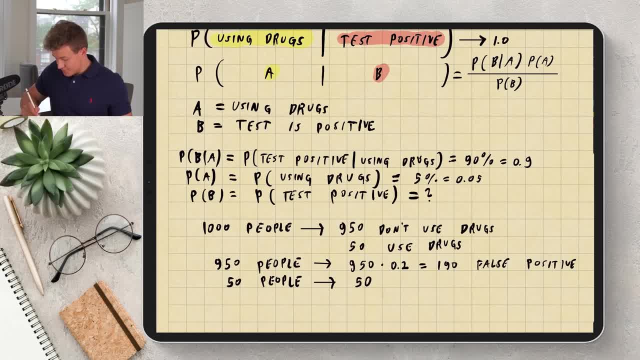 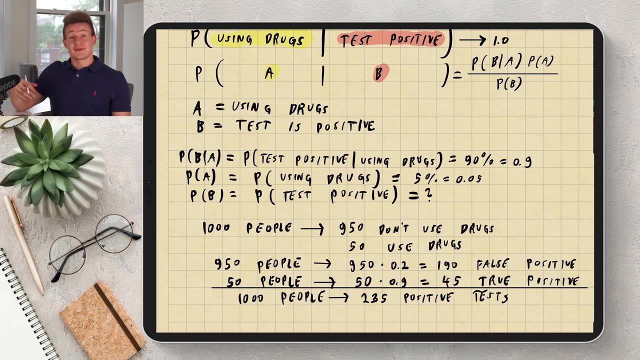 to tell us that it's positive. So all that is now left to do is add up these numbers. That is 190 plus 45, which is 235.. So we know that out of the 1,000 tests that we made, 235 of them turned positive, In other words, 23.5% of. 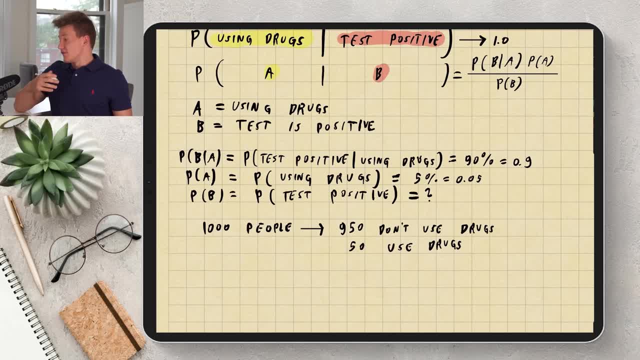 So let's first look at the 950 people. We know that the false positive tests are going to be 20%, so we just have to multiply 20% by 950, in order to get how many false positives are going to be positive. 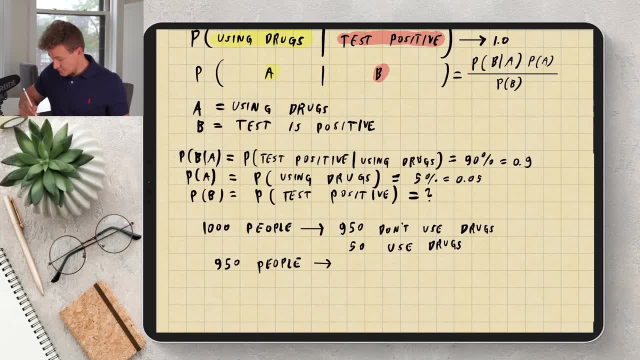 So there's a total of 190 false positive tests For the 50 people. we also know how the test behaves, Namely, we know that for 90% of the people who actually do use drugs, the test is going to trigger and it's going to tell us that it's positive. 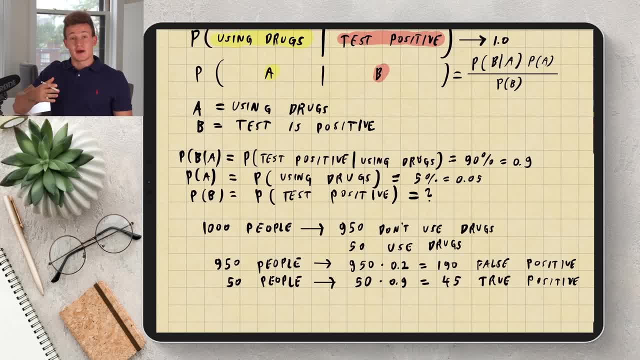 So all that is now left to do is add up these numbers. that is 190 plus 45,, which is 230.. So we know that out of the 1,000 tests that we made, 235 of them turned positive. In other words, 23.5% of the tests are positive. 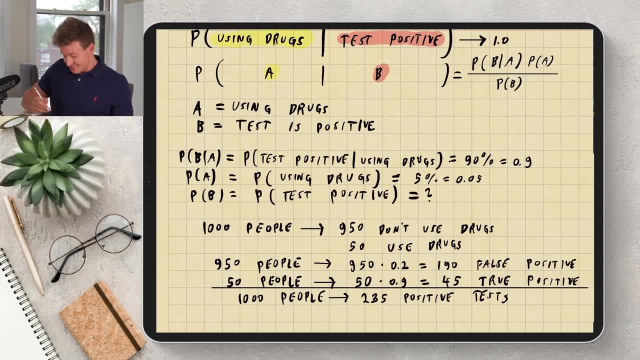 So p of b is 0.235.. That is basically it that we have to solve Now. we just have to plug these numbers back into Bayes' theorem. We are going to get a result. So overall, the answer is roughly 19%. 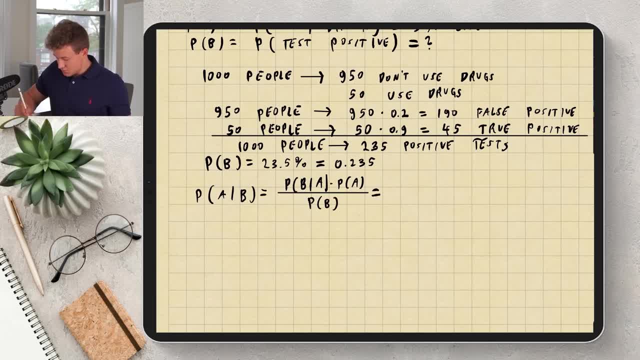 In other words, that means that only four out of five of the tests are actually correct, Meaning that for every five people that get accused of using drugs, only one of them has actually been doing it And therefore the test is really bad. 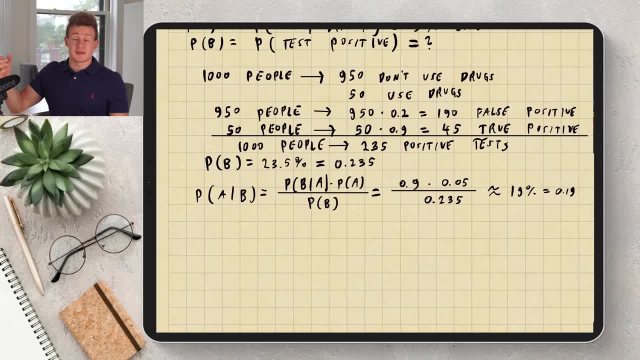 This concludes step number two. Just to summarize, step number one was really understandable and it was a really good test, So I hope you enjoyed it. If you liked it, please give it a thumbs up and I'll see you in the next video. 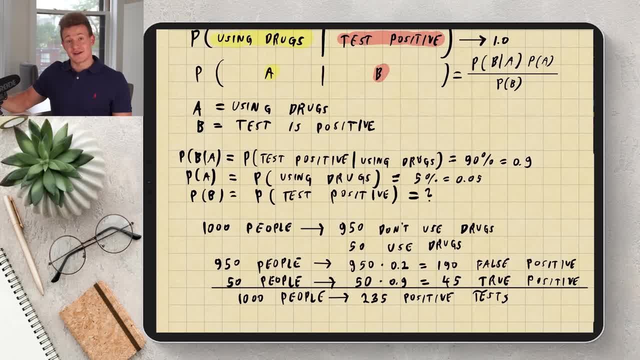 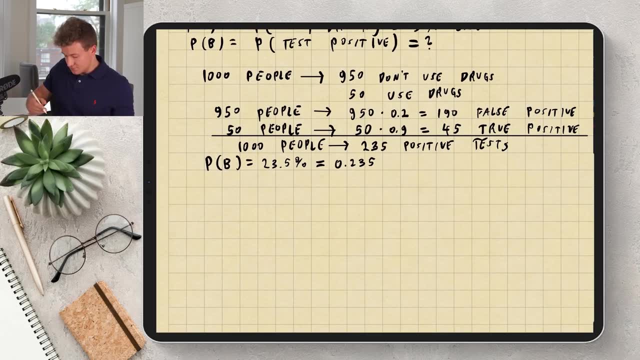 the tests are positive. So p of b is 0.235.. That is basically it that we have to solve Now. we just have to plug this in. If we plug these numbers back into Bayes' theorem, we're going to get a result. 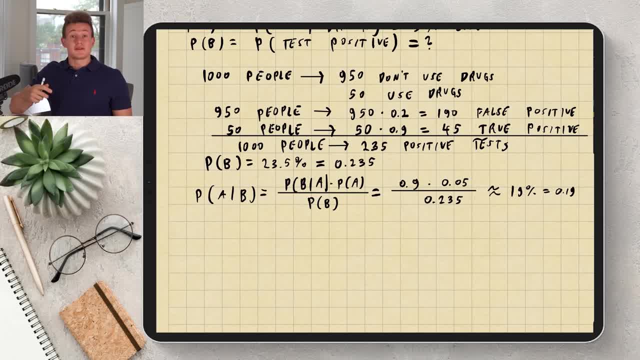 So overall, the answer is roughly 19%. In other words, that means that only 4 out of 5 of the tests are actually correct, Meaning that for every 5 people that get accused of using drugs, only 1 of them has actually been doing it. Therefore, the test is really bad. 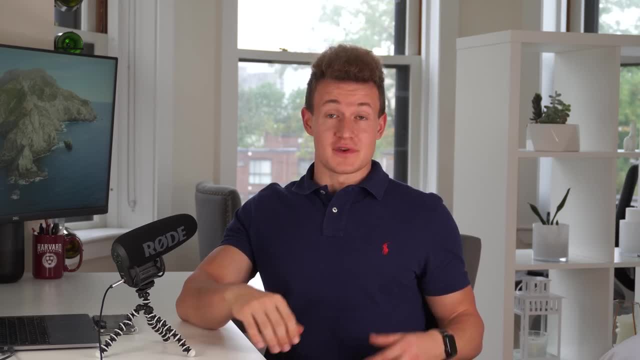 This concludes step number 2.. Just to summarize, step number 1 was really understanding the problem and analyzing every aspect of it, And step number 2 was talking to other people and explaining to them everything you know about the problem so they can challenge you. 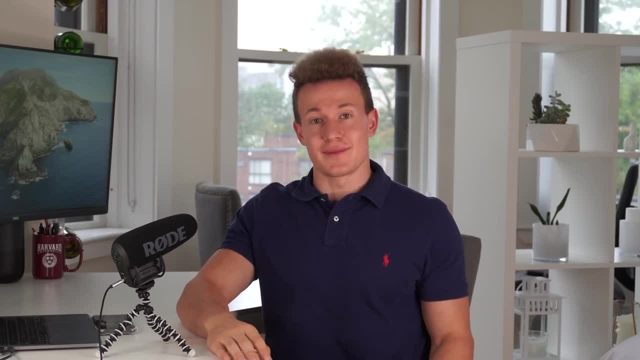 in everything you say. Also, you should always break down the problem into sub-problems. Step number 3,, according to Feynman, is write down your solution. This may sound a bit silly and I personally haven't written down many solutions for many years, and I deeply regret. 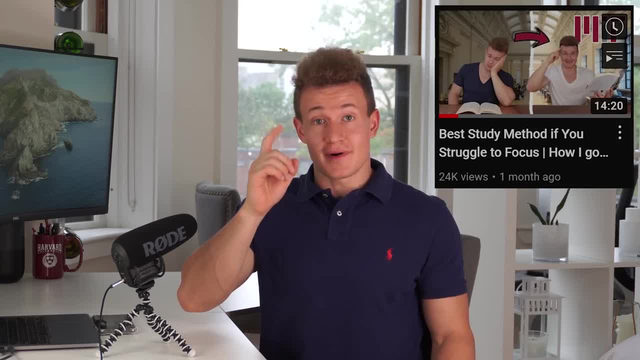 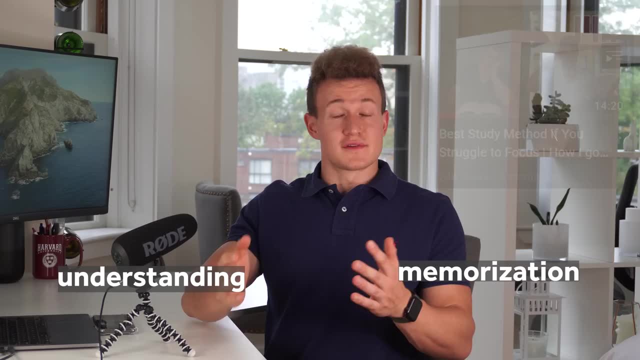 it. As I explained in my video about the best study methods, there are two parts to learning something: Memorization and understanding. You often make the mistake thinking that, for example, geography or history is all about memorization, and math and physics is just. 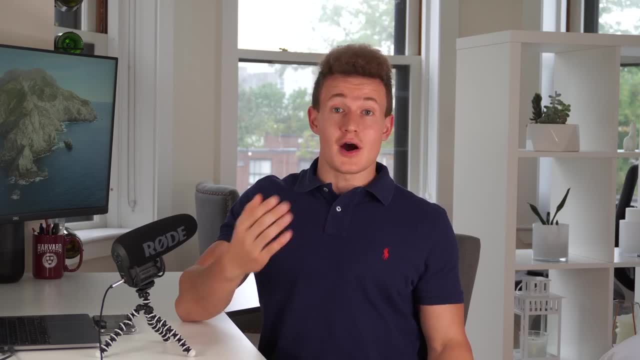 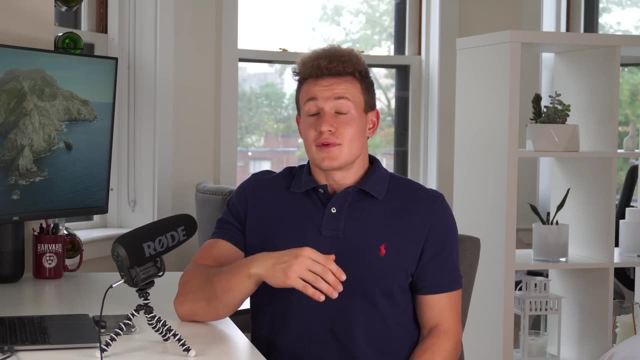 about understanding something, But this is completely wrong. Understanding a complex concept may be a great mind exercise, but in the end of the day, if you do not remember what you understood at some point in the past, you will not be able to use that skill in. 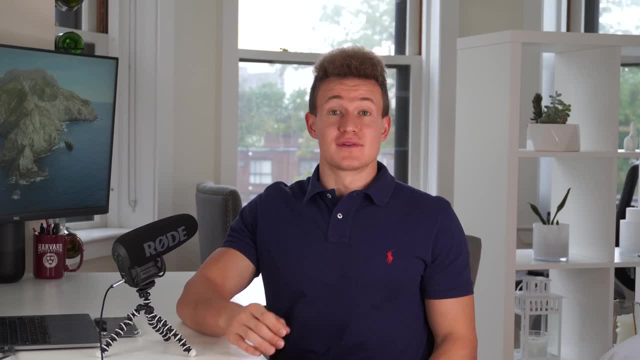 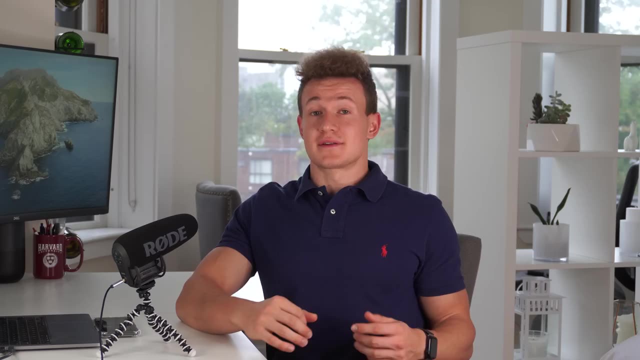 the future. I personally learned so many advanced mathematical tools in university and I really understood them during my exam, But then after the exam I would never really write them down and nowadays I really regret that I actually forgot most of them. so I can't really 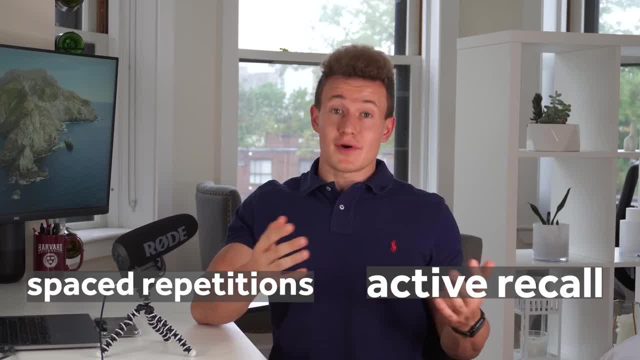 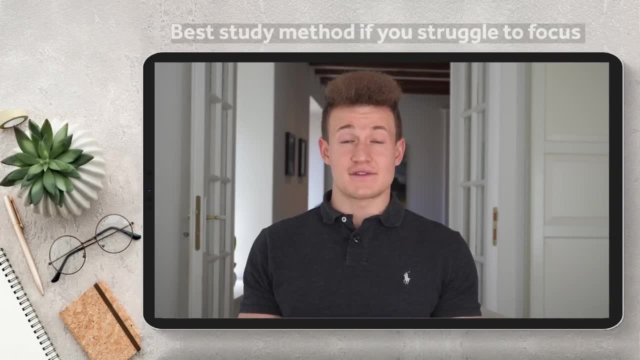 use them. The active recall and spaced repetition techniques allow you to memorize things for life. So, after watching this, make sure to check out my video on spaced repetition and active recall techniques. The solution to my struggles, which drastically changed my life in so many ways, came from: 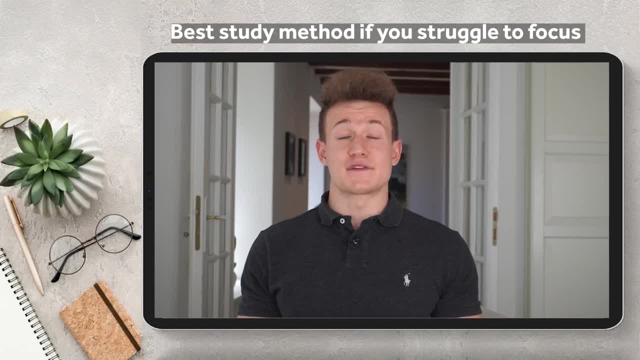 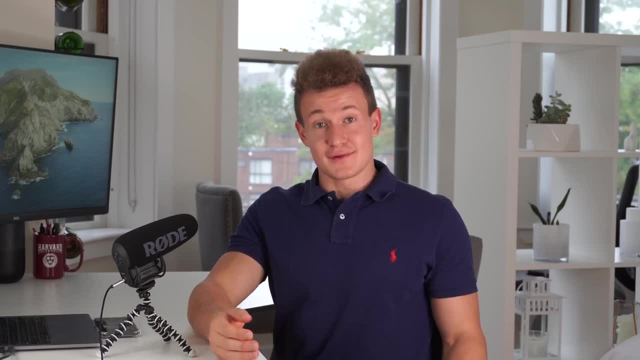 my mom. One day in 10th grade she came to me and told me about a software called Anki. Anki is the only software for which I would seriously say that it changed my life. This concludes step number 3.. With Feynman's principle for solving problems, I'm now going to give you a few tips and tricks. 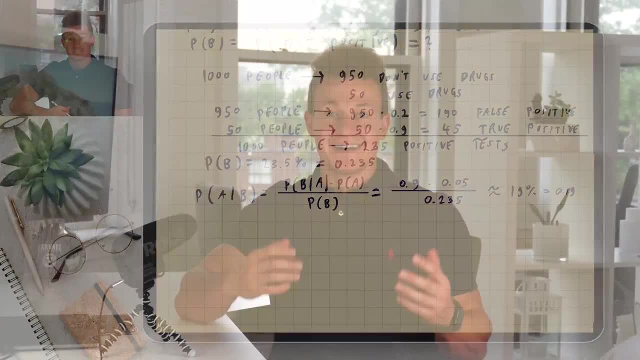 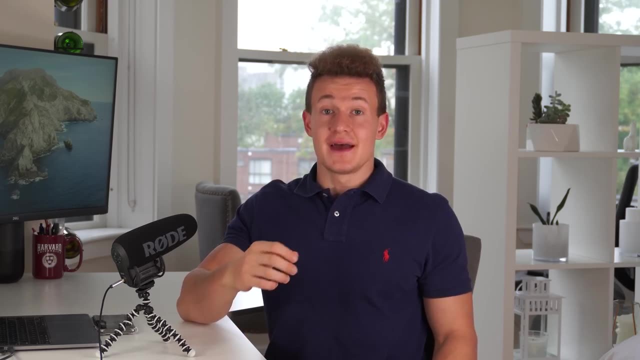 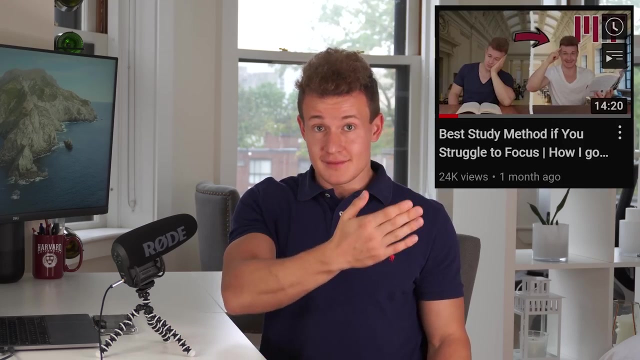 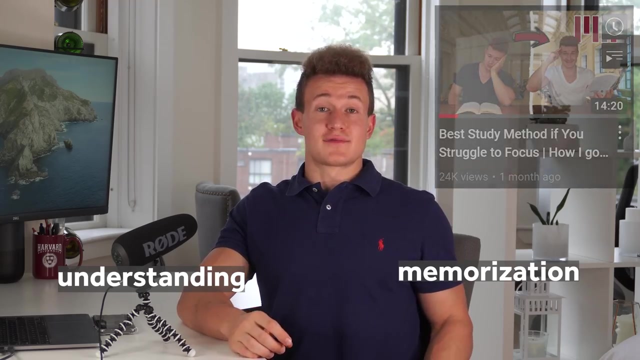 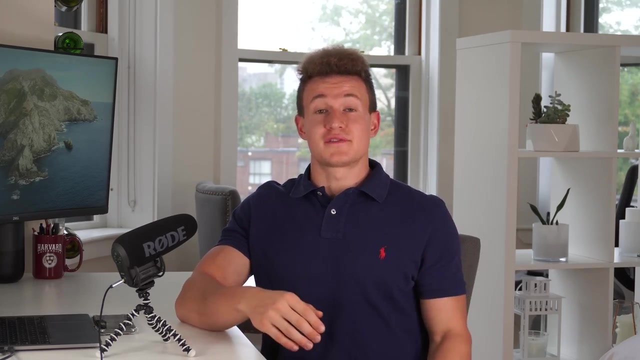 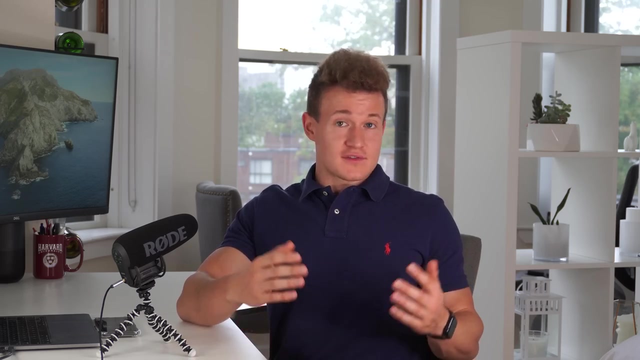 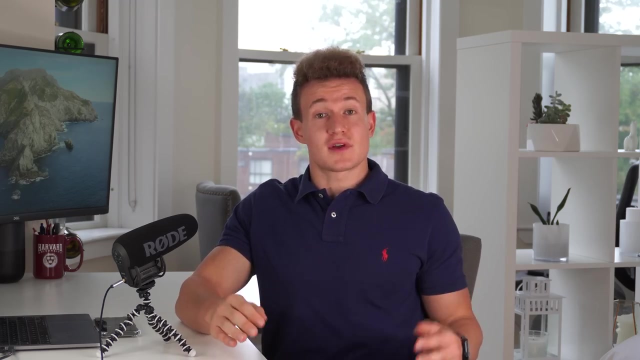 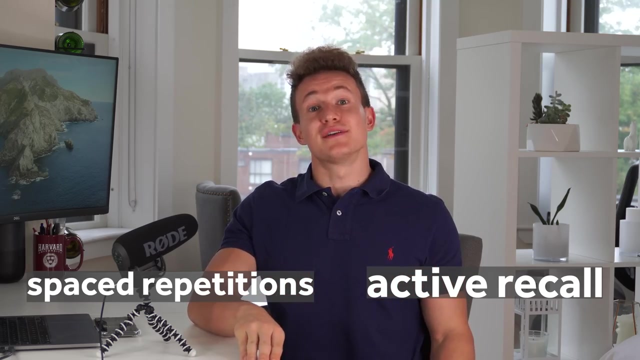 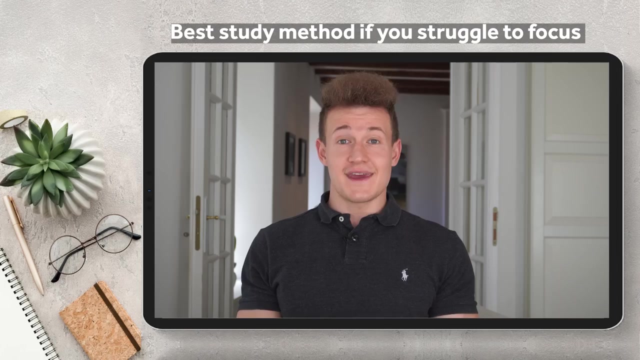 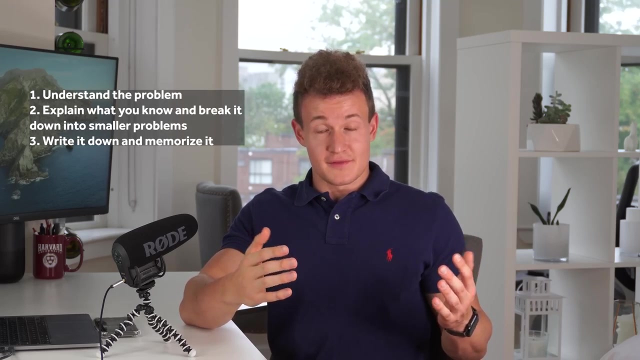 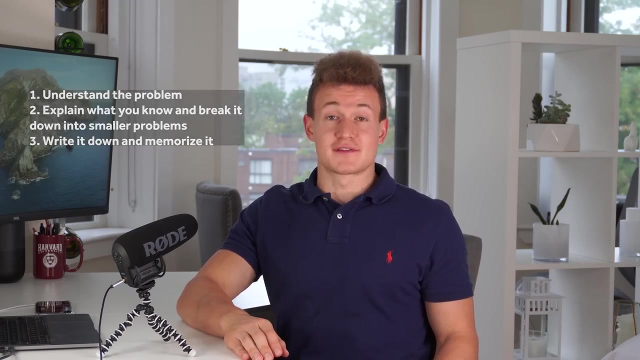 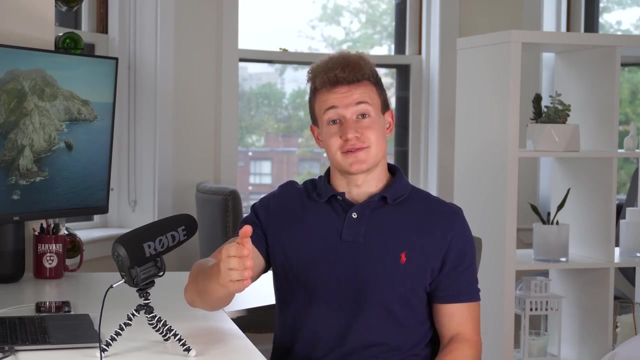 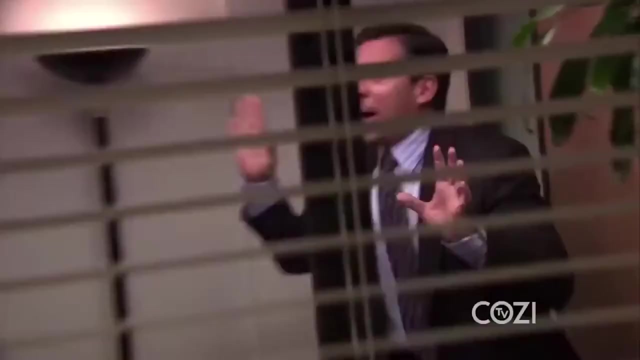 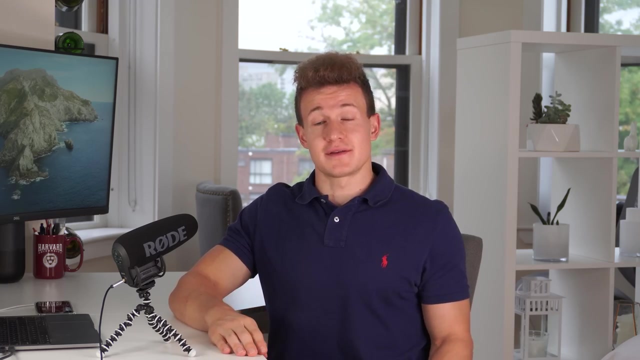 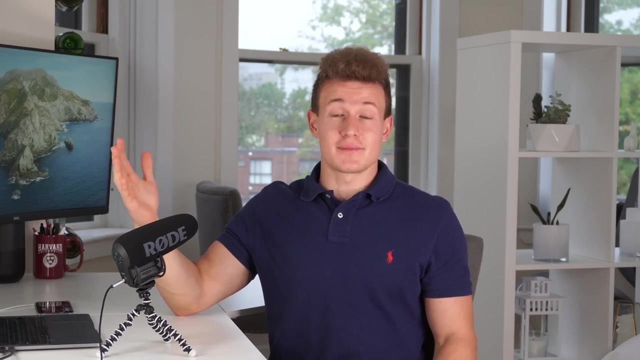 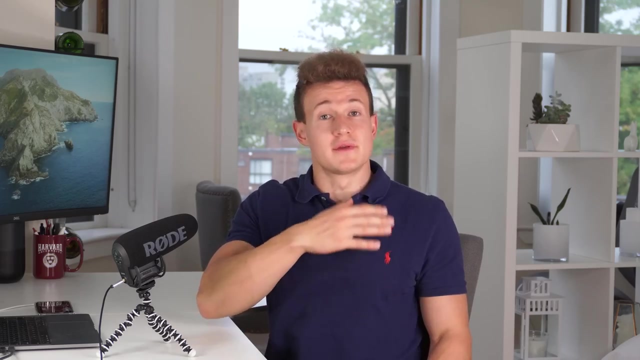 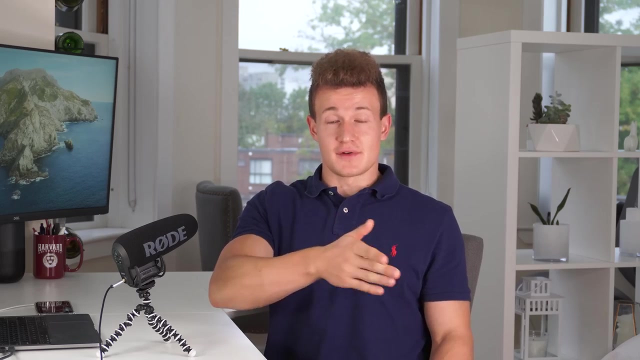 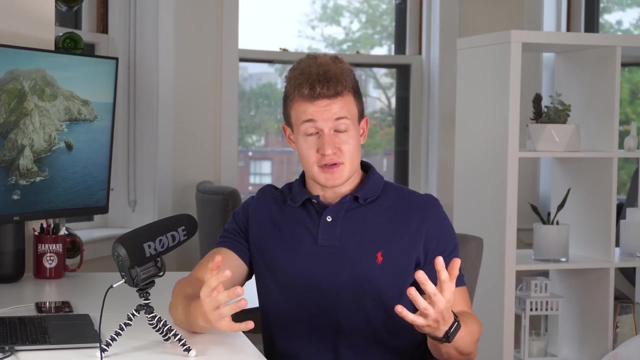 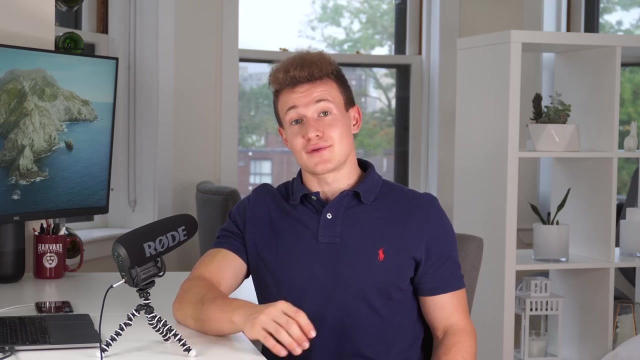 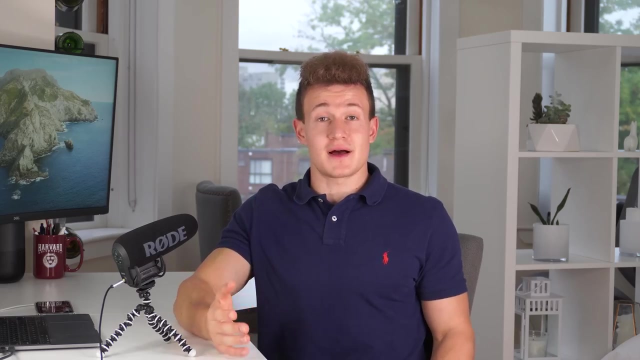 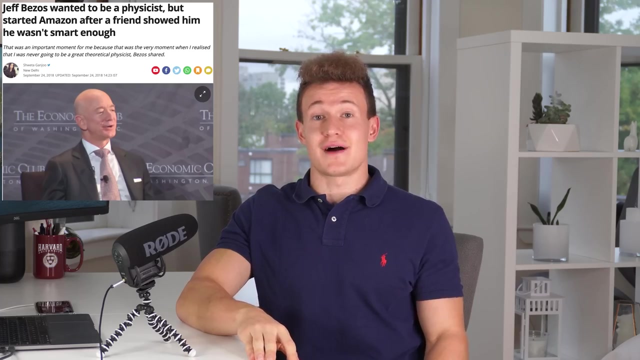 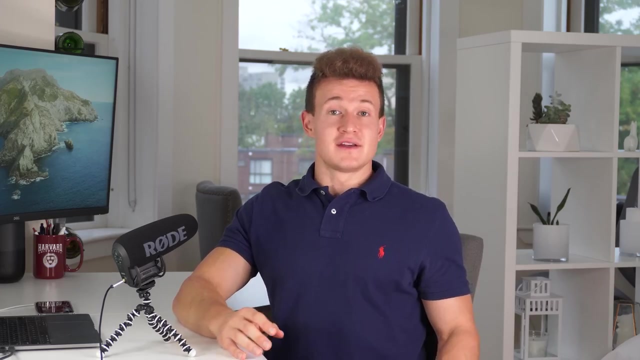 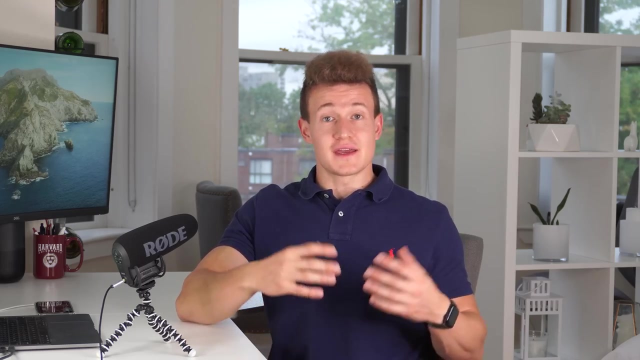 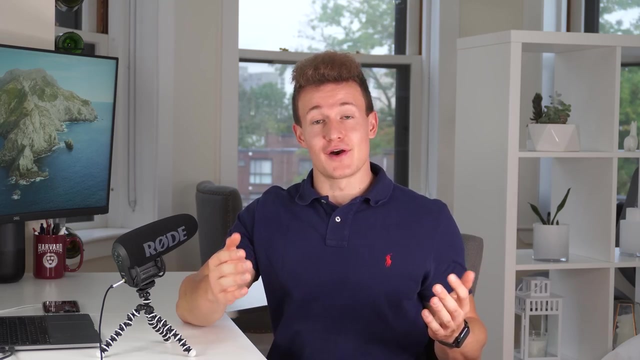 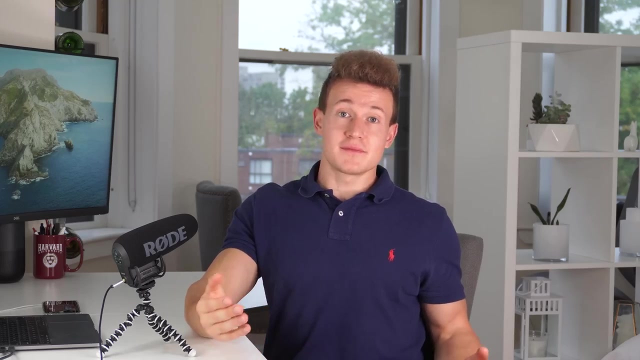 Bye. Subtitles by the Amaraorg community: wwwamaraorg, wwwamaraorg, wwwamaraorg, wwwamaraorg, wwwamaraorg, wwwamaraorg, wwwamaraorg. 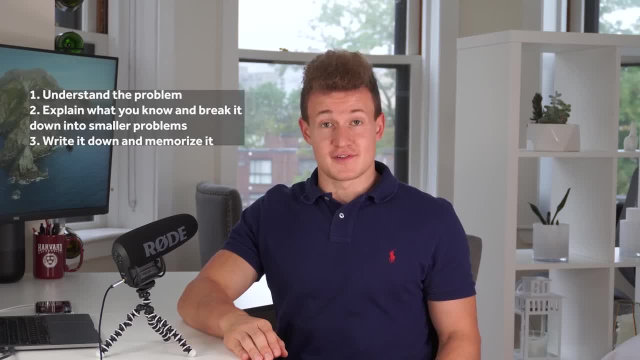 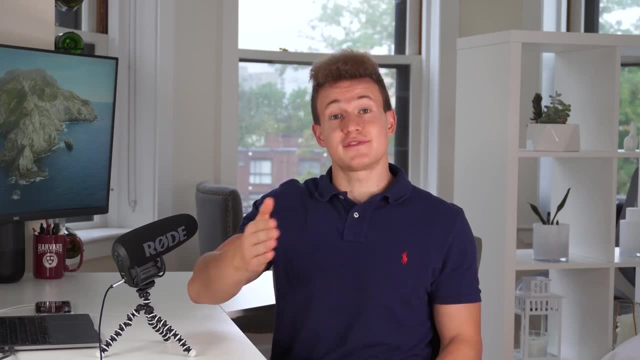 which I use throughout my life. One of the major reasons why a lot of people struggle solving complicated problems, especially if they're under time pressure, is because they don't manage to stay calm and just follow their problem-solving procedure. Oh my god, Okay, it's happening. Everybody stay calm. 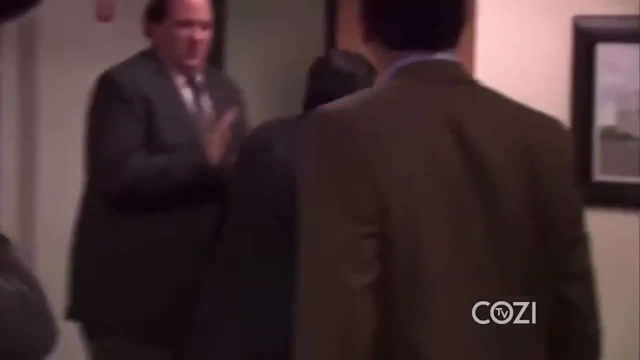 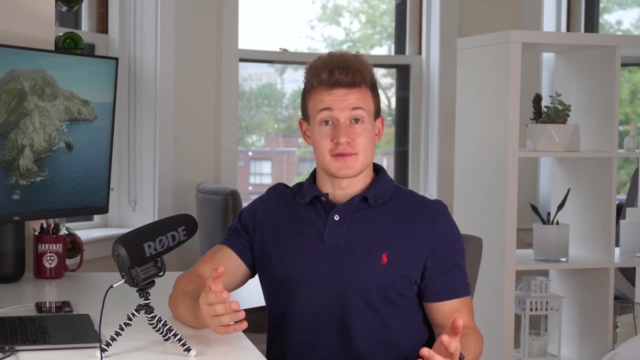 What's the procedure? everyone? What's the procedure? Stay f***ing calm, Wait, wait, wait, wait. At the International Physics Olympiad, I would sometimes be confronted with incredibly complicated problems that took several pages just to explain. Panicking and just daring these problems. I would just calmly follow Feynman's procedure. 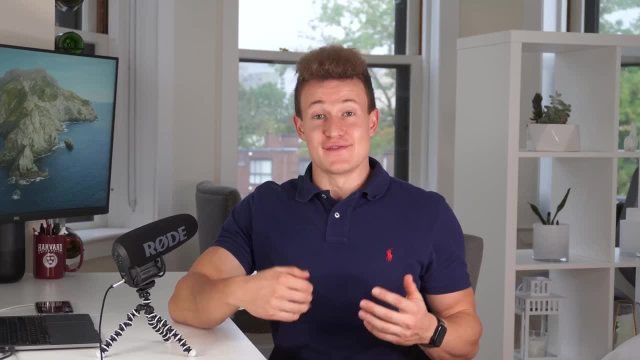 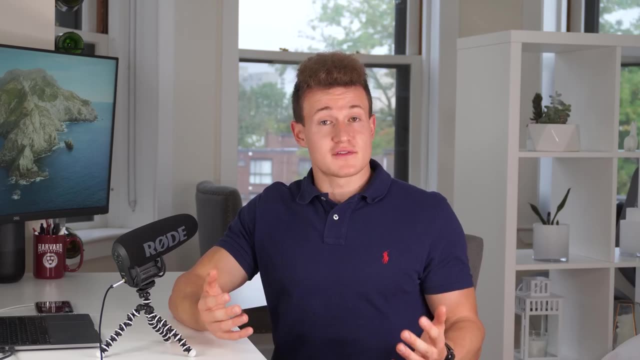 for solving problems and after some time I would end up with a solution. If you're still having difficulty solving certain problems, at least in mathematics, science and maybe engineering, you can apply the following tricks If you struggle solving some kind of analytical problem or a problem that has very messy numbers. 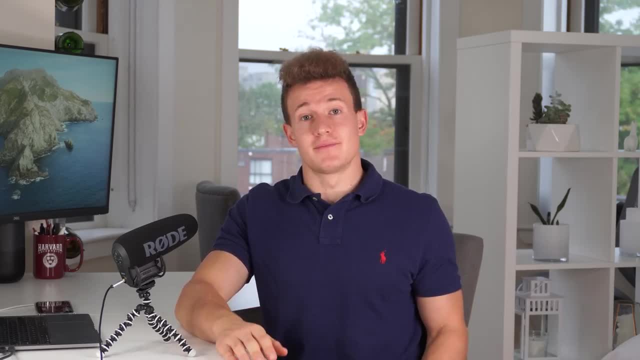 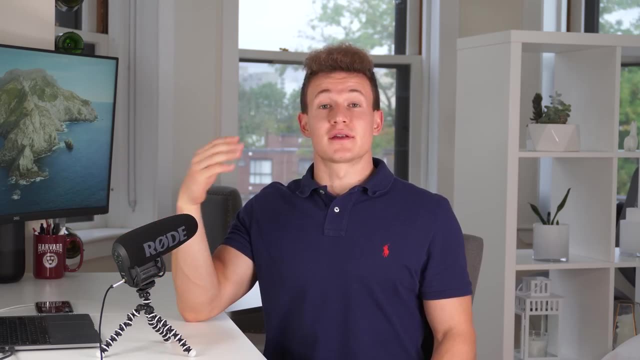 you could, for example, replace all of them with one and try to visualize the entire problem. Some problems are just too complicated because they have so many variables, so by setting some of them equal to zero and solving the problem first, you can understand it, and 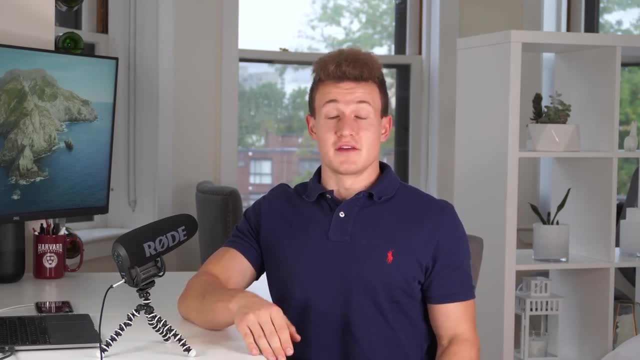 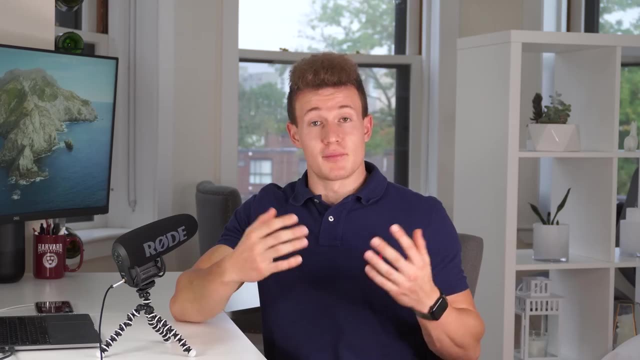 then you can always come back and solve the original problem. Or, instead of making variables equal to zero, you can simply remove some of the information from the problem and then write it down in a more simple way. If you don't know how to approach a certain problem, maybe you've solved a similar problem. 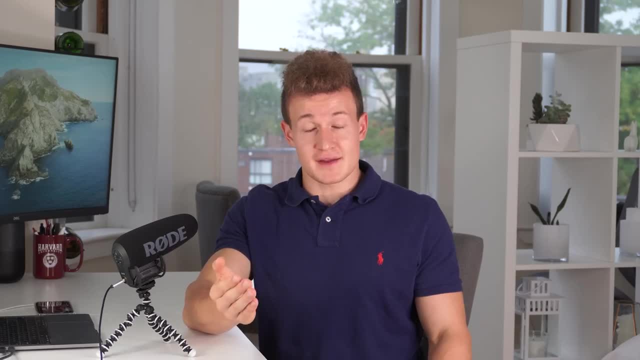 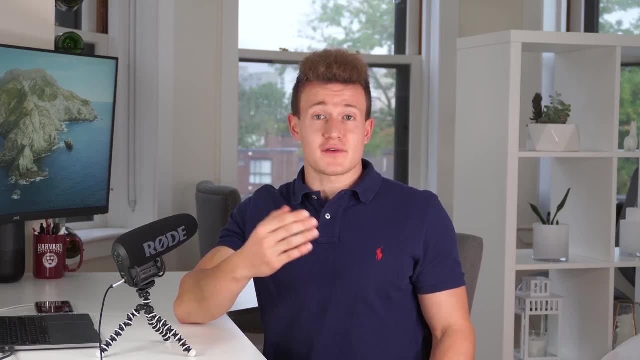 in the past. so first have a look at that. figure out how you solved that, and then maybe the solution will become obvious. Jeff Bezos once wanted to become a theoretical physicist. that's why he was studying at Princeton, and he was really stuck with that problem for many hours. 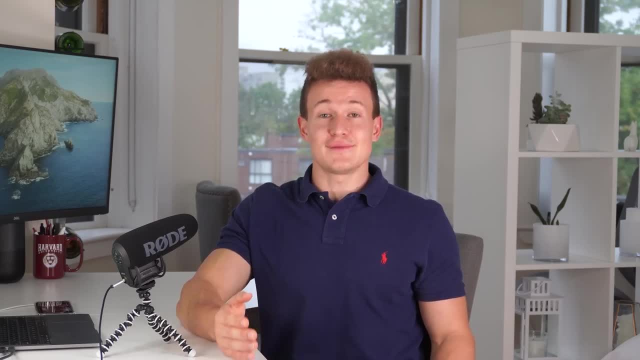 He then just walked up to a friend and was like: hey, I don't really know how to solve that, can you help me? And his friend just looked at the problem. he could tell him the solution on the spot. When Bezos asked him how exactly he did that, his friend simply replied: oh yeah, it's a. 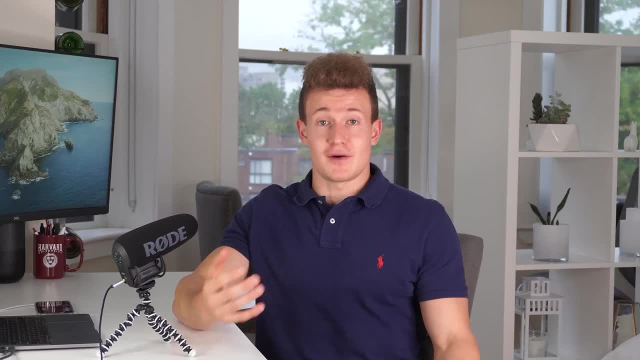 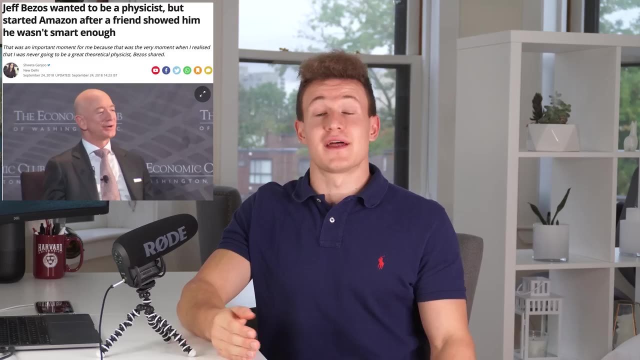 bit similar to another problem that he saw in class and therefore the solution was obvious. And Jeff Bezos was so discouraged by the fact that he simply couldn't comprehend this that eventually he gave up on doing physics and started Amazon. Also, if your first attempt to solve a problem didn't work, don't try again the same way. 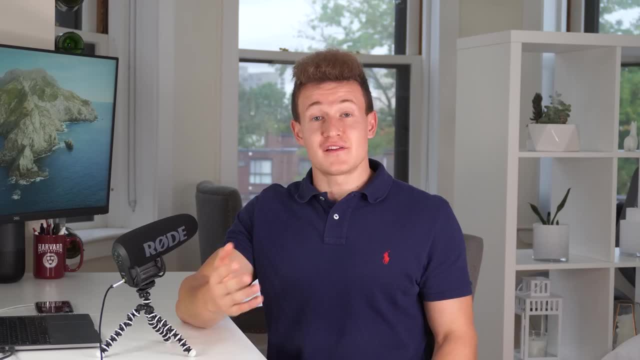 Try thinking about other ways you could approach this problem. Quantum mechanics itself was probably the silliest possible solution to explain all the inconsistencies in physics in the early 20th century, but yet it turned out to be true. These were my strategies for understanding and solving complex problems.